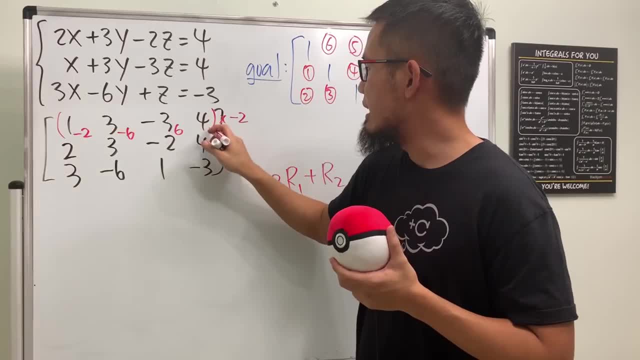 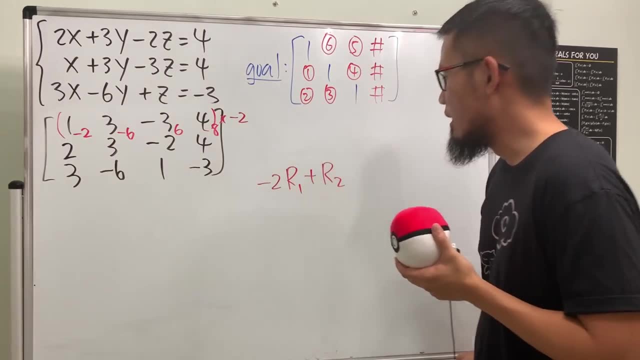 Negative 2, negative 6, and then 6, and then negative 8.. It's easier for us to see when we combine right. I think that will be better, in my opinion. But again, follow your instructor if you are, you know, taking a linear algebra class. 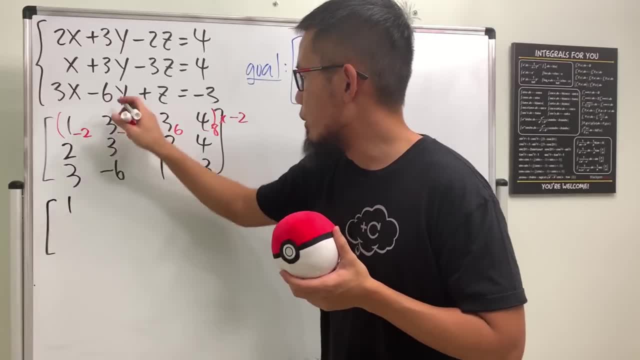 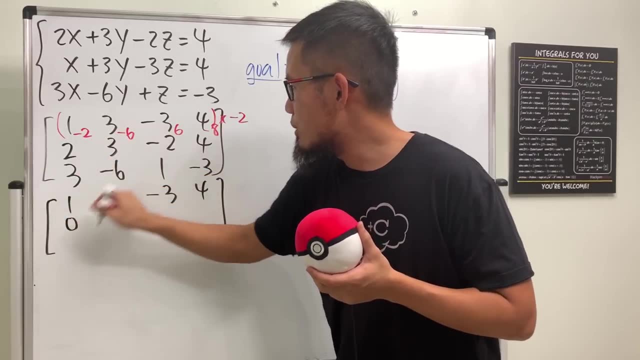 All right, The first row stays because we haven't done anything with it. We're just writing as 1, 3, negative 3, and 4.. So combine this and that together, we get 0.. This and that together, we get negative 3.. 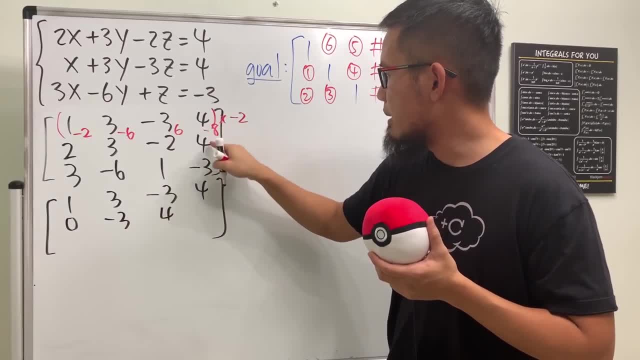 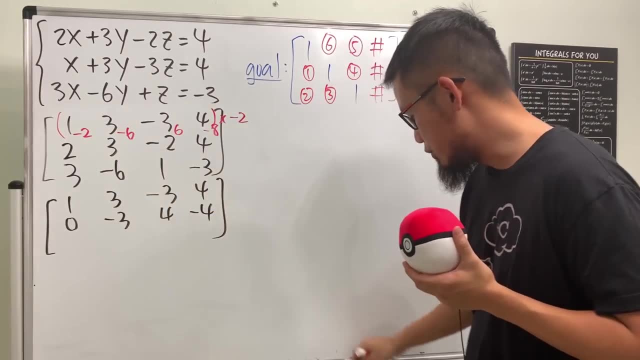 And then pass the 4.. Negative 8 plus 4 is negative 4. Like that. And now I want to make this equal to 0.. Here we have positive 3.. So I'm just going to take this row again and I will multiply it by negative 3.. 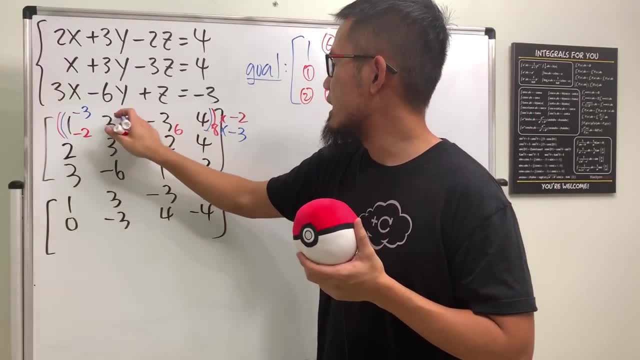 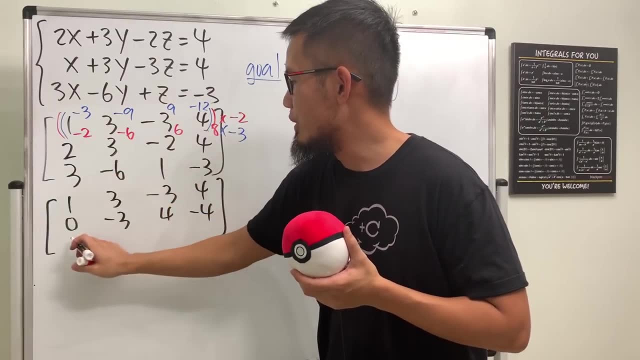 This time I'll put down the result right here: We get negative 3,, negative 9, positive 9, and negative 12.. Have a look: This and that together, we get 0.. This and that together, we get negative 15.. 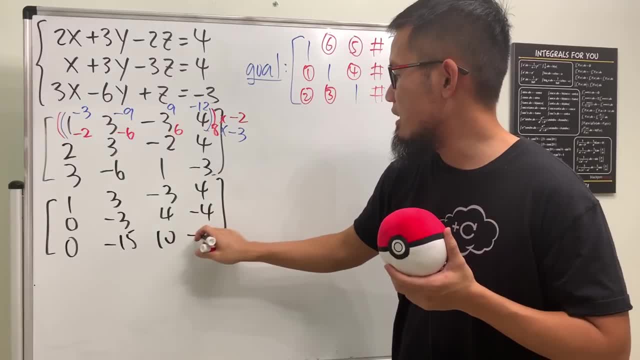 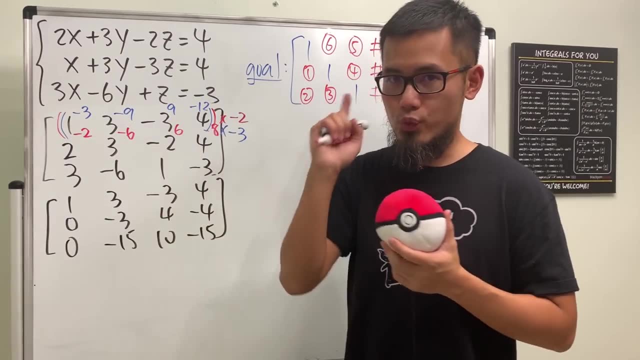 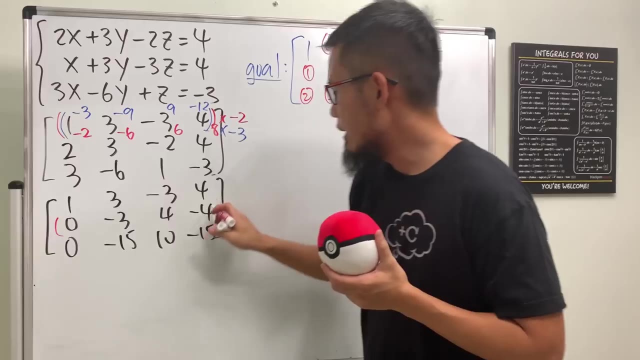 And then 10. And then negative 15.. Just like that. So the first column is done. Now we want to make this entry equal to 1.. So what we can do is: here we have negative 3.. We can just take the second row and divide it by negative 3.. 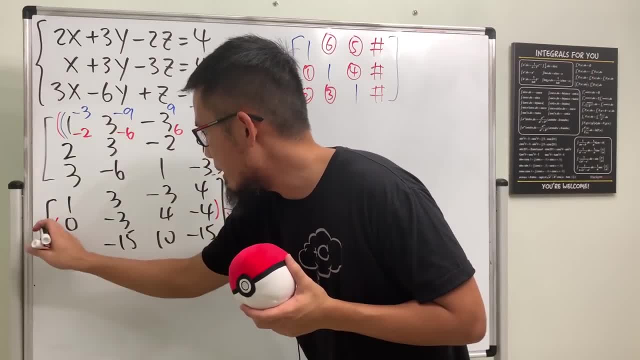 We'll multiply by 1, third, Same thing, right, And again the first row will stay the same And technically you should draw arrows like this. And then let me just write down: 1,, 3, negative 3, and 4.. 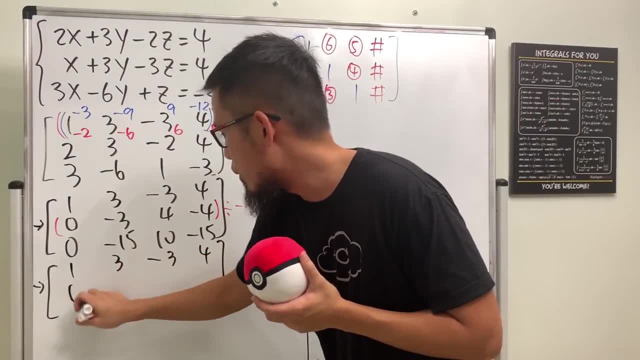 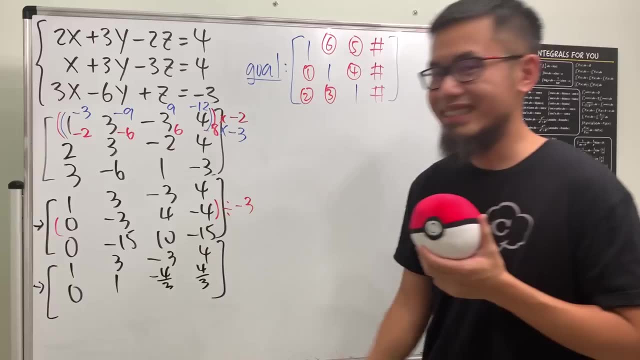 Second row, we have 0,, 1.. And this and that is negative: 4 over 3.. And this and that together is positive 4 over 3.. Alright, good, Now here we want to make this equal to 0.. 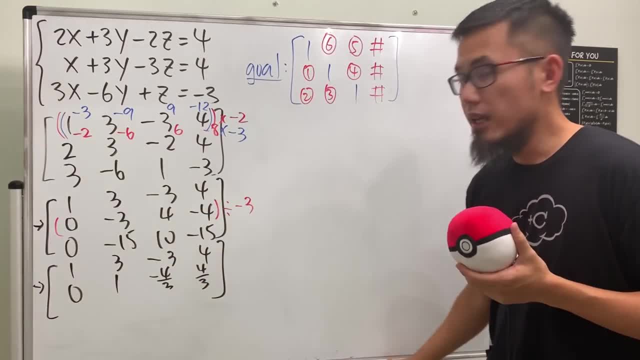 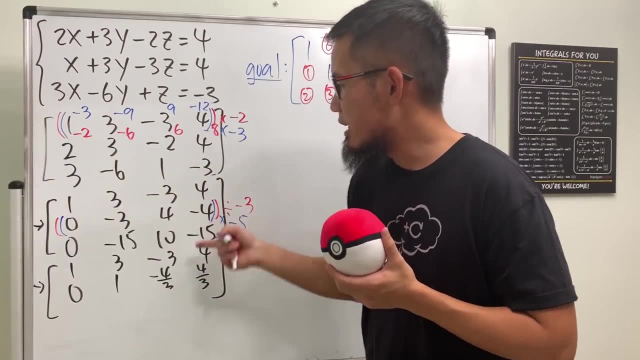 In fact, I will use this row as how it is, So that I can actually just multiply by negative 5.. 0 times negative 5 is just 0, so that doesn't matter. This and that together is positive 15.. 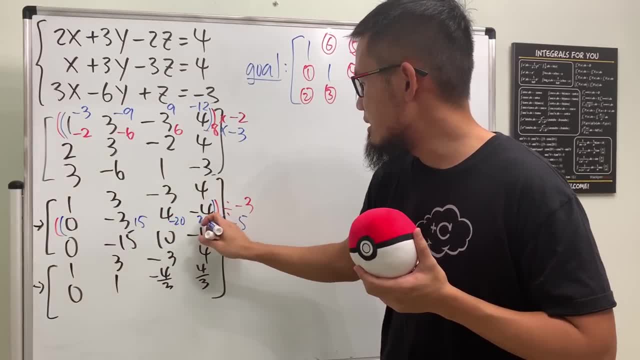 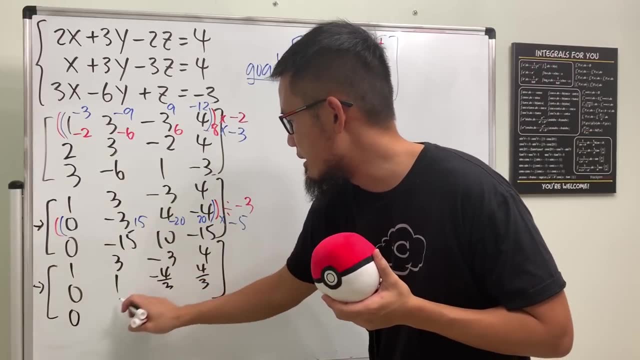 And then negative 12. And then negative 20. And then, lastly, this is positive 20.. Alright, so just combine. So 0 and 0 is 0. And this and that is 0. This and that is negative 10.. 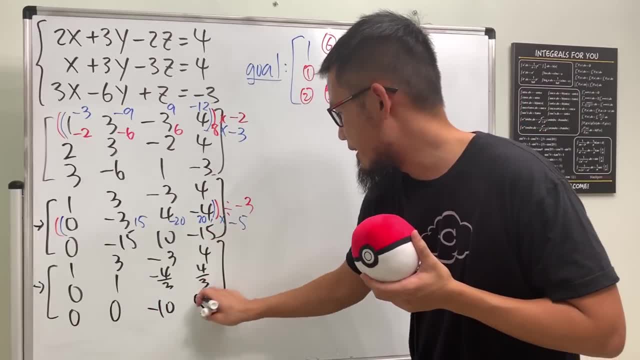 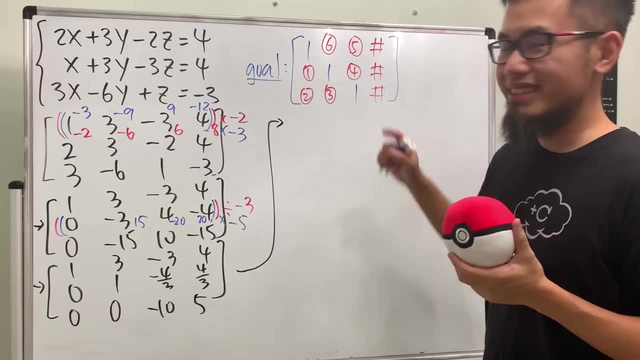 And this and that is positive: 5. Like that Cool Now. so far, so good. right, We want to make this equal to 1.. This is negative 10. All we have to do is just take the last row. 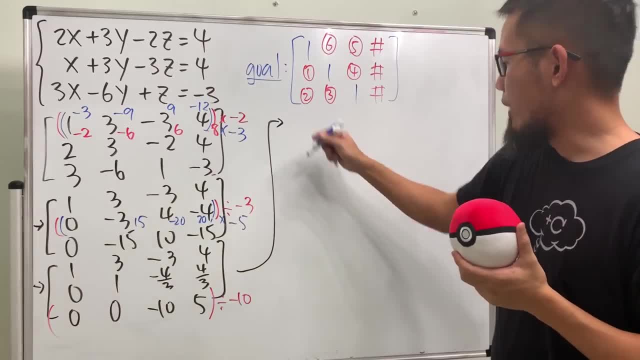 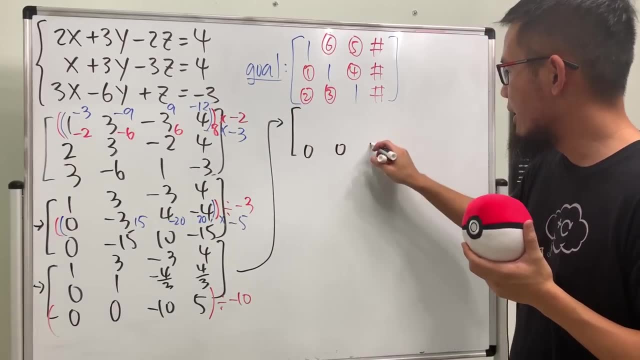 and divide it by negative 10.. So from here we will actually write down the last row first. So the last row, we get 0,, 0,, 1.. And this and that becomes negative 1 half, Like that. 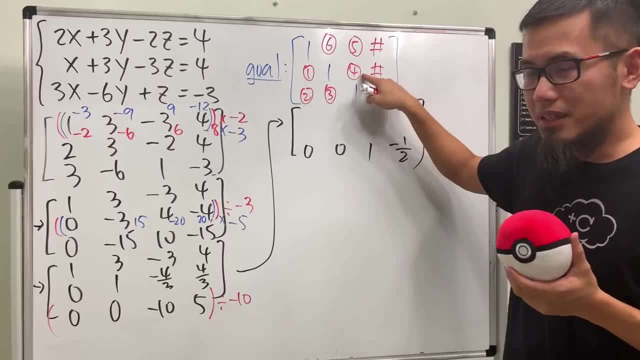 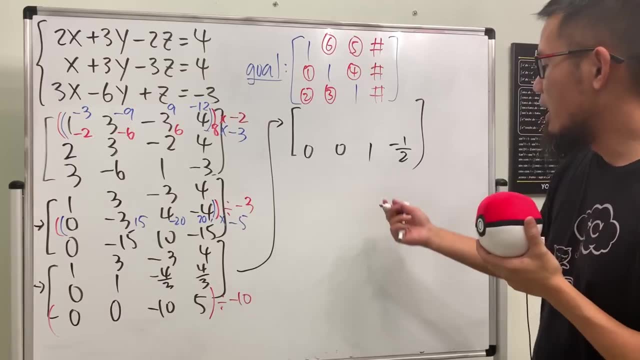 Okay, then just continue. I want to make this equal to 0.. And I will actually use this row right here. What I can do is, because this is negative 4 over 3, let's just multiply this by positive 4 over 3.. 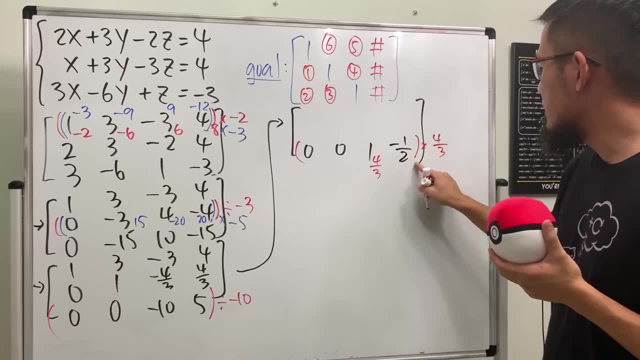 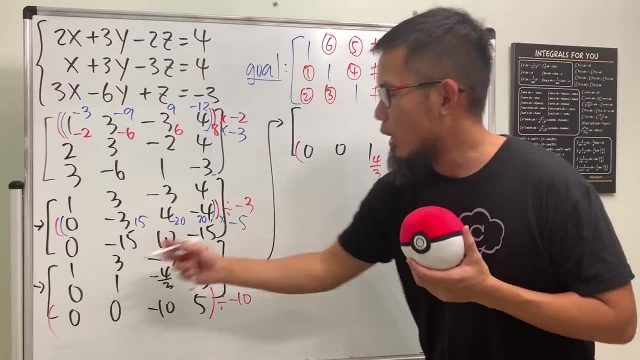 So we get positive 4 over 3.. And this and that we get negative 2 over 3, after you reduce, And then you take this, add it to them And we end up with 0,, 1, and 0.. 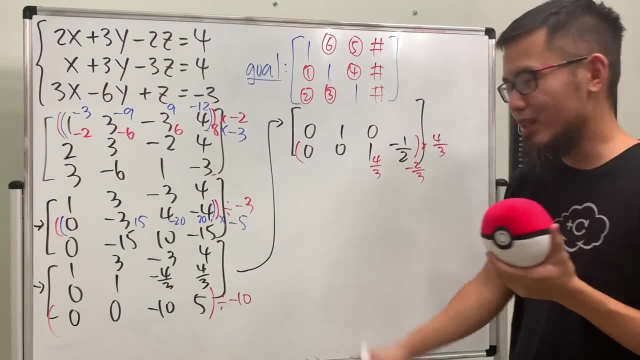 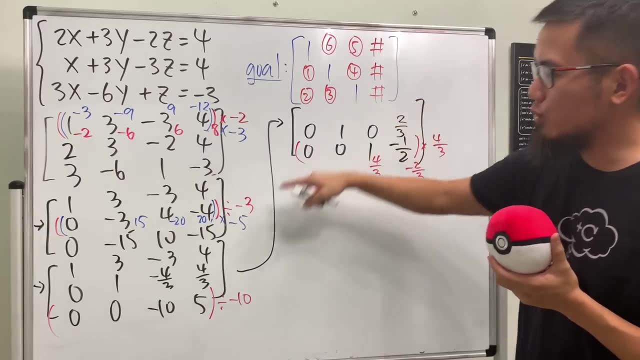 Negative: 2 over 3, and this is positive 4 over 3.. They have the same denominator already, which is very nice. We get positive 2 over 3.. Okay, so we got that done. Now we want to make this and 3 equal to 0. 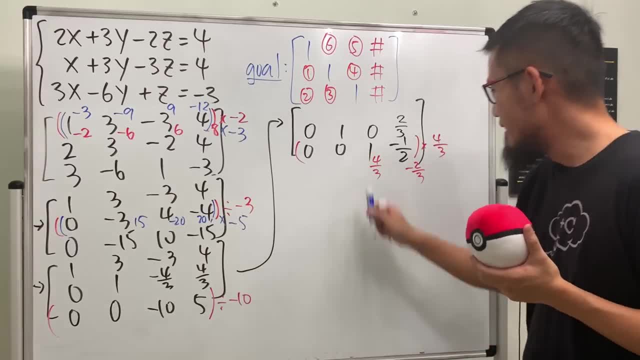 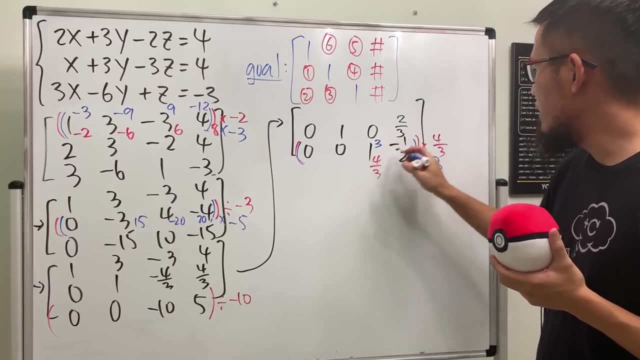 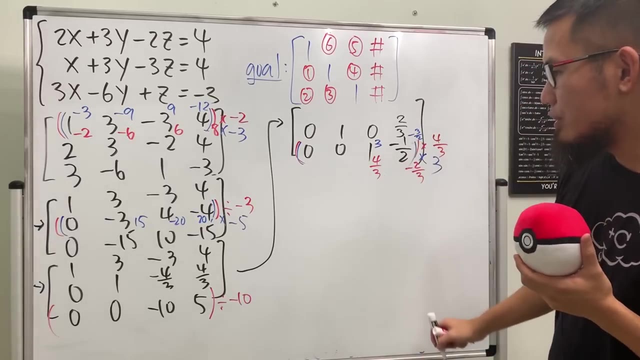 And we have negative 3.. So I will take this thing right here again. multiply this by positive 3.. So here we get positive 3, and this becomes negative 3 over 2.. Alright, Now I'm just going to add these numbers to them. 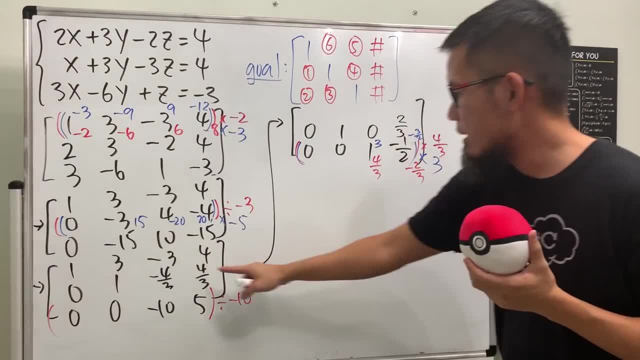 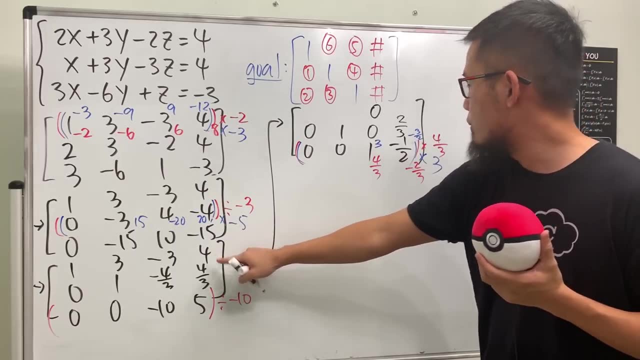 This and that, actually this and that becomes just 0. And this is negative 3 over 2 plus 4,, which is the same as 8 over 2.. So we get positive 5 over 2.. And then we still have the 3 and 1,. 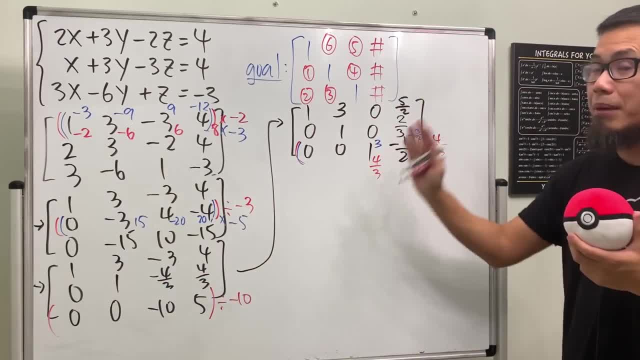 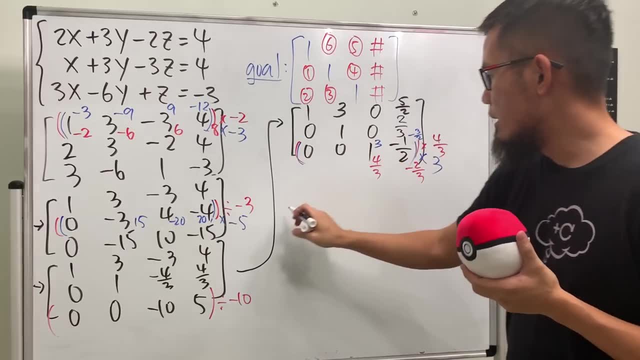 reading backwards like that. Okay, so just pay attention to the numbers in black. Lastly, we just need to make this entry equal to 0.. And we will have to use a second row, Alright, So I'm just going to keep the last row as how it is. 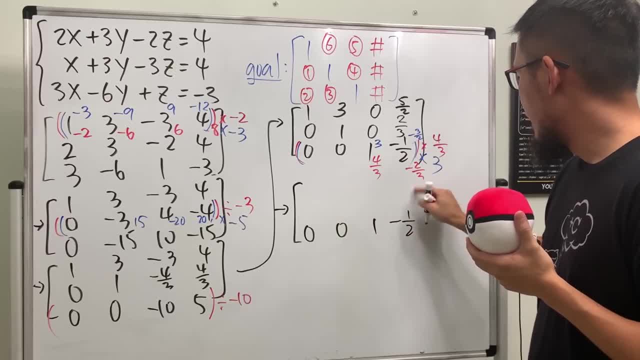 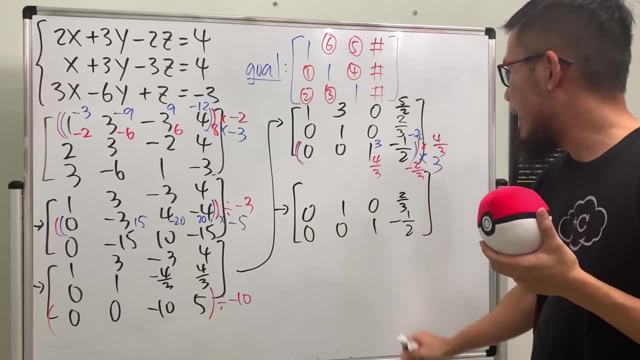 0, 0, 1, and negative 1 half, And then this row stays the same as well: 0, 1,, 0,, 2, third. But for this row I will actually take it. 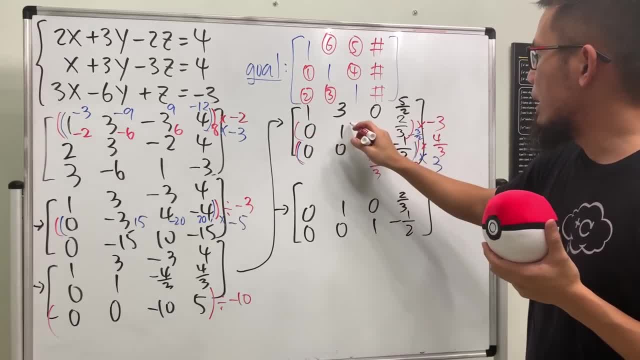 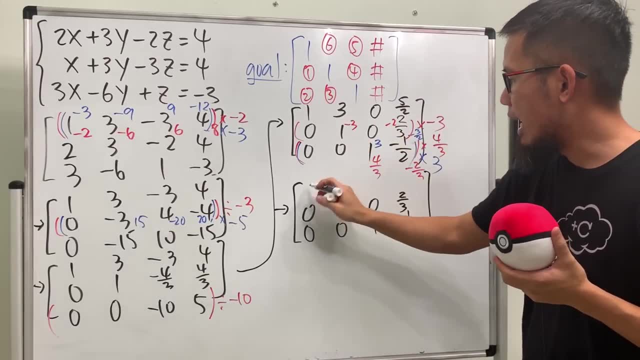 and then multiply it by negative 3. And I will get negative 3. This right here is negative 2.. And then I will just add these two numbers to them, So I get 1, and then this, and that is 0,. 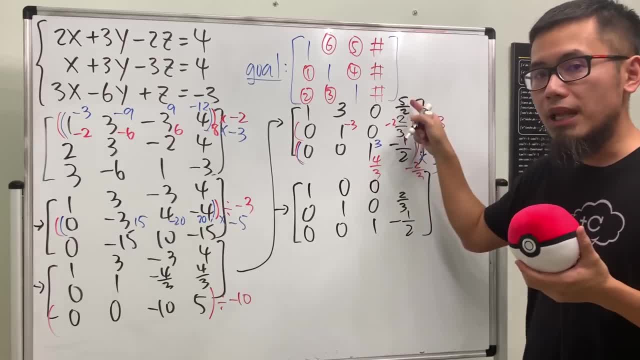 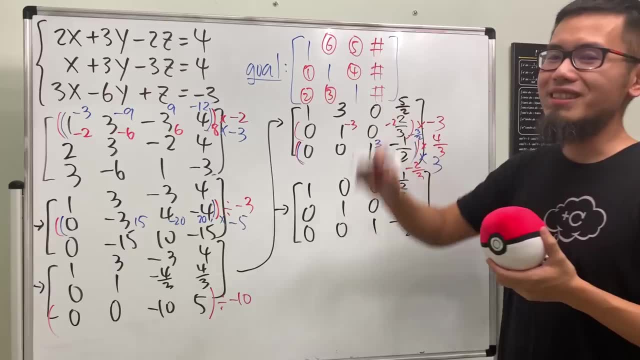 and this is still 0.. Lastly, negative 2 plus that is negative 4 over 2 plus that. So we end up with positive 1 half. So, as you can see, we achieved what we wanted, Right? So in this case, 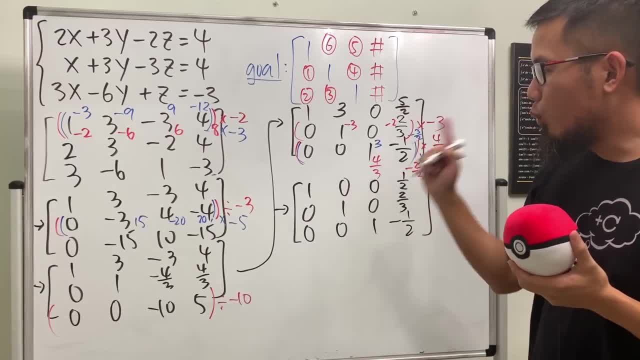 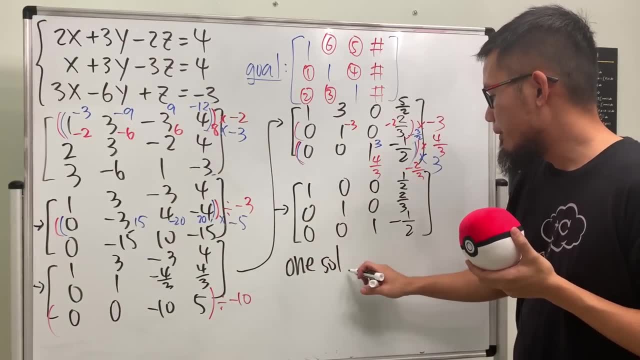 well, I will write down the answer for you guys. We have actually one solution situation whenever you have 1, 1, 1 like this. So one solution, one unique solution. And then let me just tell you the intersection. 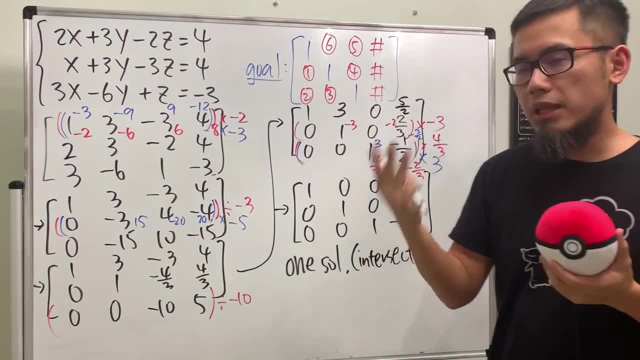 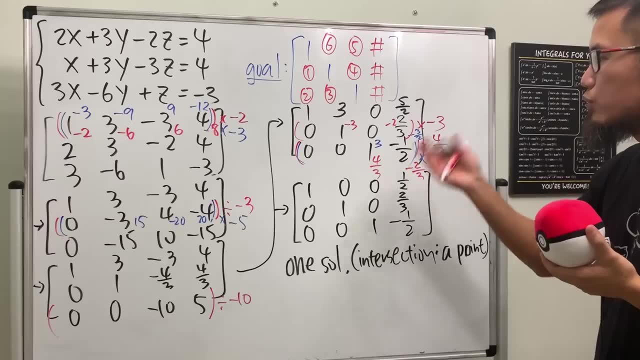 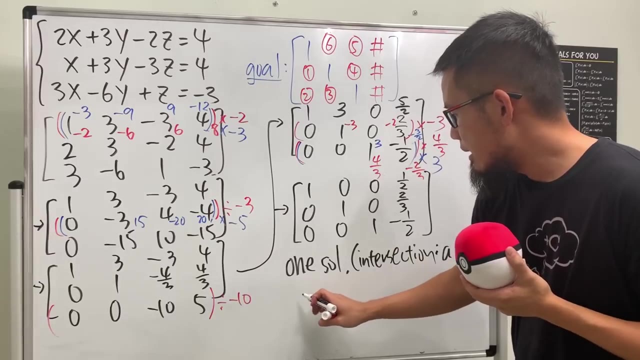 of all this right here, and you see this right here are just three planes in the space. The intersection is just a point. Whenever you have just one solution for that, three planes intersect at one point, Very nice. Okay, And how can you write this solution? 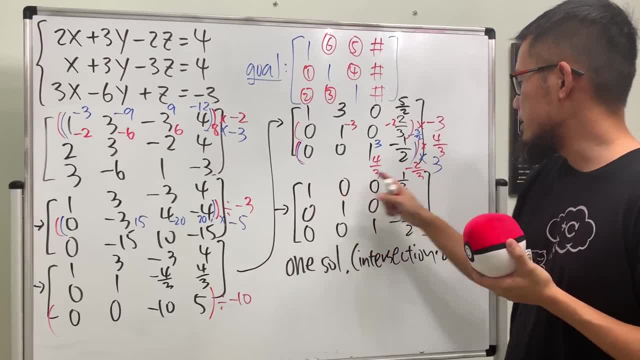 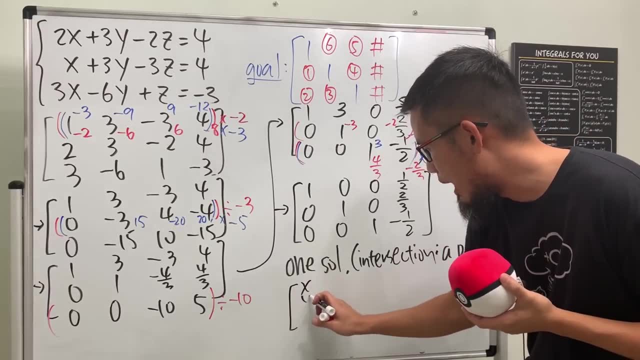 Depends on your teacher or depends on whoever You can write down: x is equal to 1 half, y is equal to this, z is equal to that, Or you can also put it in the factor form x, y, z, And I think this is how I'm going to present the answer for you guys. 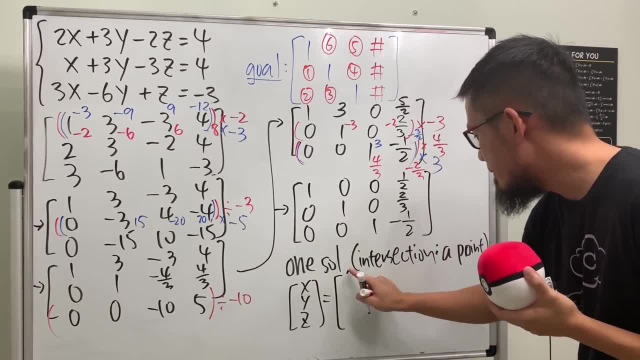 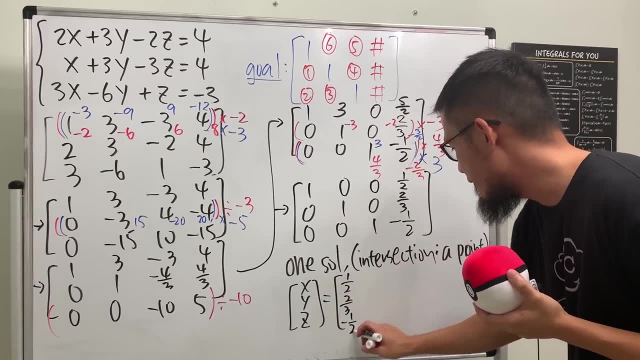 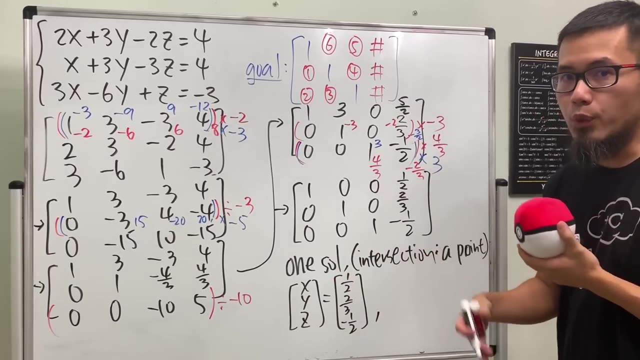 x, y, z. x is 1 half And then y is 2 third And lastly, z is negative 1 half. Just like this. And notice that when you have one solution, this right here, we actually do not have what we call the free variable. 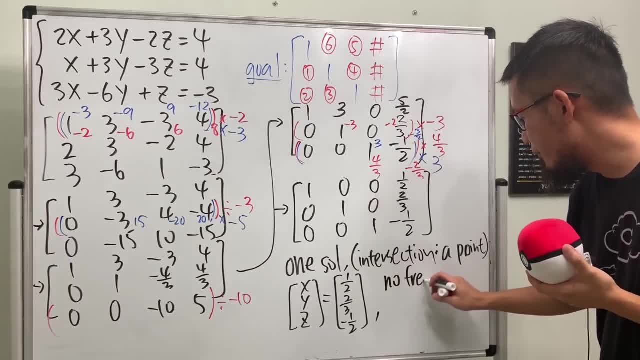 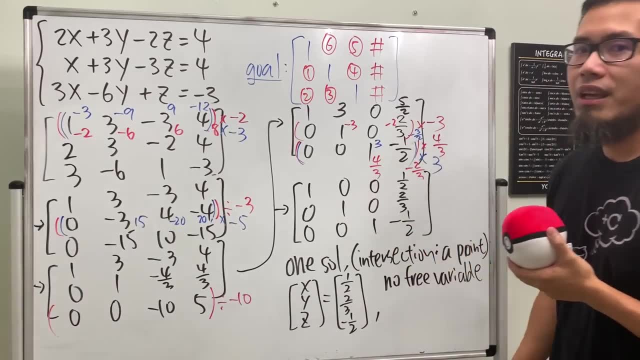 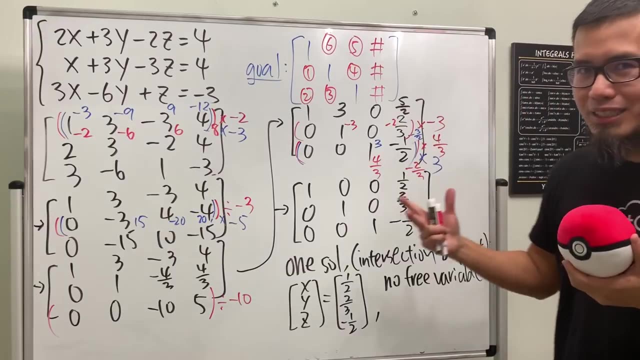 So let me just make a note right here: No free variable in our situation. I will demonstrate the free variable in the next example. And one last thing is that whenever you have one solution to your system, at least one right. Sometimes you have a lot, infinitely many. 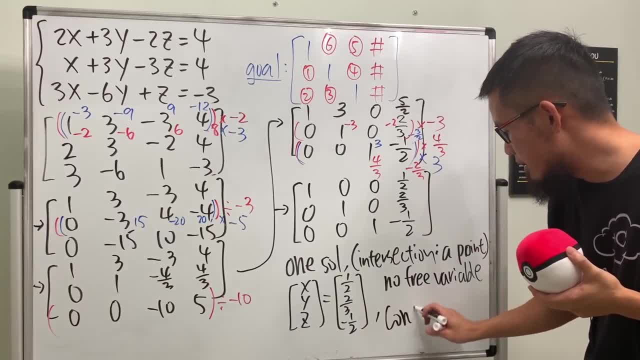 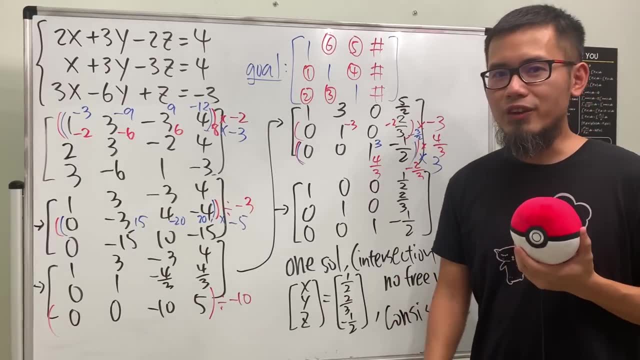 You call this right here consistent. This is a consistent system of equation. So just kind of know the terms of that stuff. I think that's one of the hardest part of linear algebra, because there are so many definitions that you have to know right. 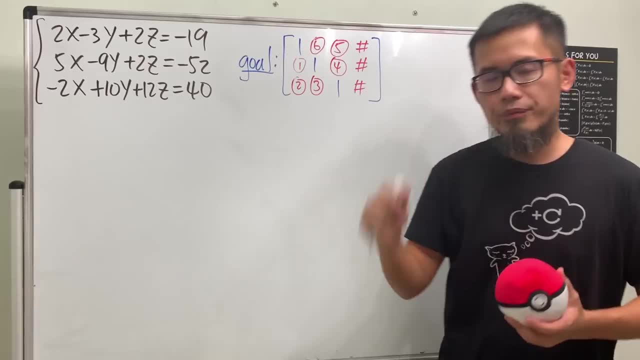 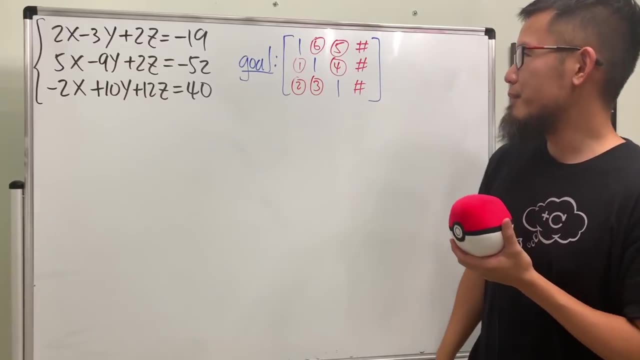 So that's the first example. Now let's take a look of the second one. So for this situation, we still want to end up right here, right? But let's take a look. what happens right here? First off, 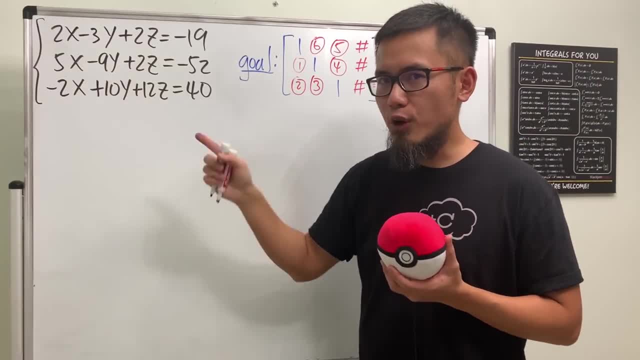 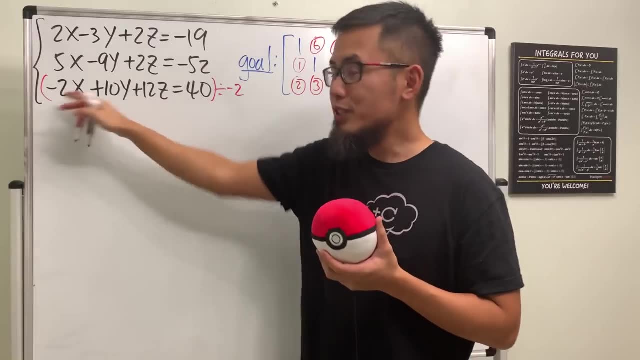 I'm actually going to write this down first, And in the meantime I will actually divide everybody by negative 2. Why? Because this way I do end up with the one that I want And also we don't end up with fractions. 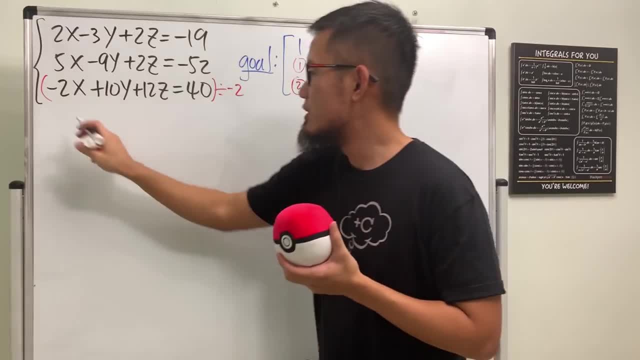 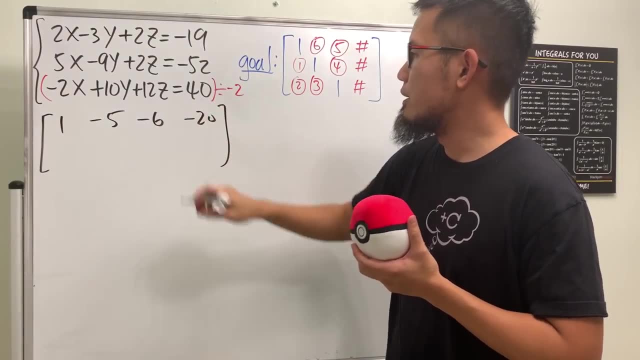 So that's why I want to put this down as the first row, right? So here we go. We will have 1, and then negative 5, and then negative 6, and then negative 20.. Okay, perfect. 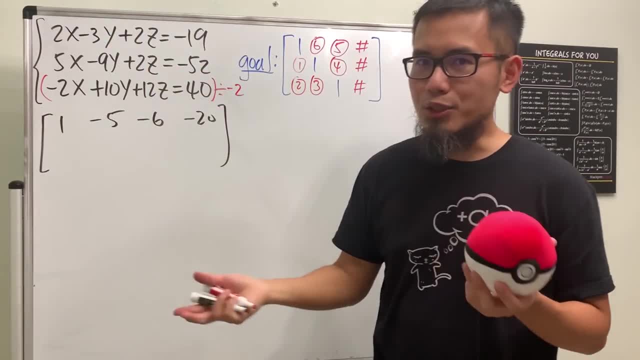 Now you know we can actually just put this down right here, But let's just save some time because you know that we will have to make this right here 0.. So let's make that happen right now. Okay, have a look. 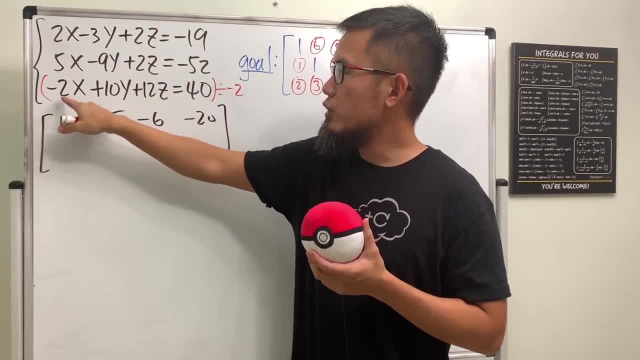 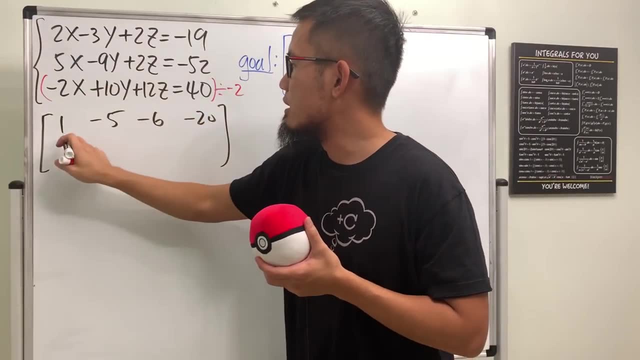 If I want to make this equal to 0,, well, we can just combine this and that together and then just put down the result right here. Let's do that Negative 2 plus that is 0, and then this and that is 7,. 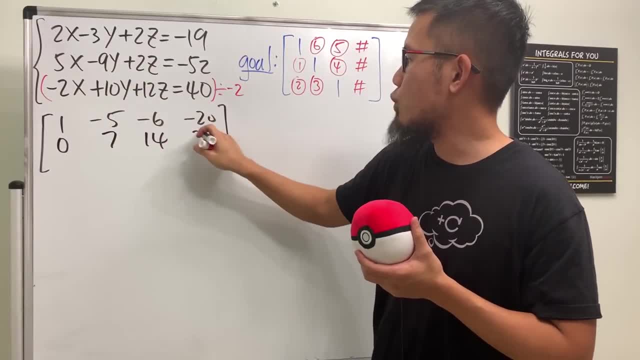 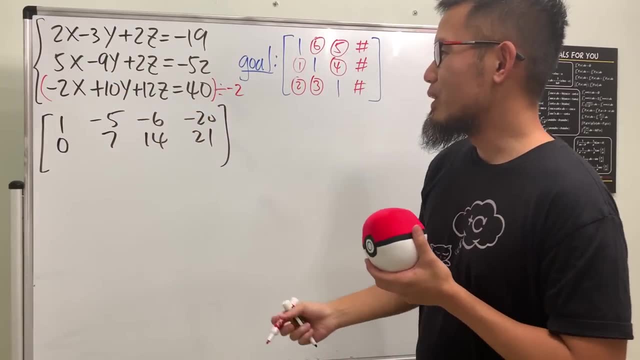 this and that together is 14, and this and that is 21.. Okay, And then, lastly, we want to kill this 5, and put it here right, And what we can do is I'm actually just take this row. 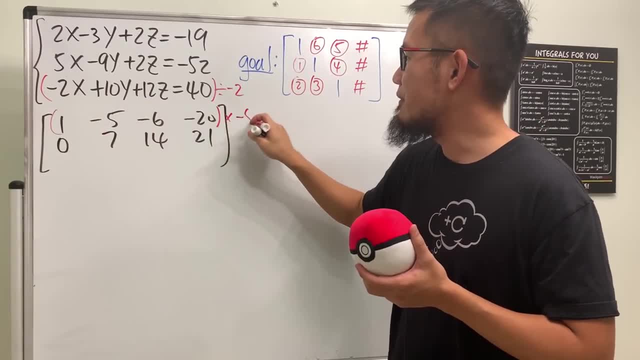 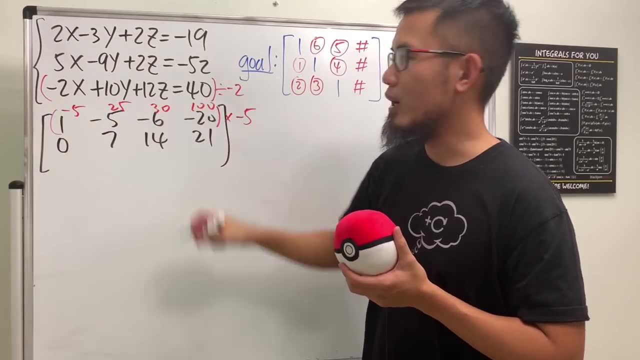 and then I will multiply it by negative 5.. Have a look: We will end up with negative 5,, positive 25,, positive 30, and then positive 100.. And I will just combine this to that which is 0,. 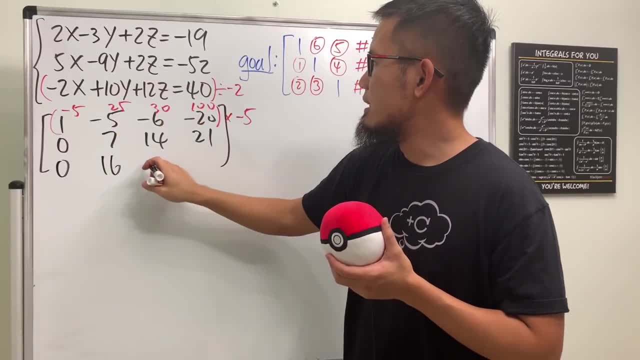 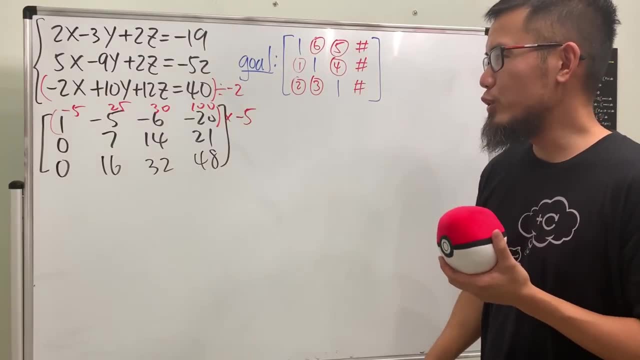 and then 16,, and then 32, and lastly we have 48.. So that's what we have. So it depends on your teacher. If your teacher really wants you to write everything down as a matrix first, then go ahead and do that. 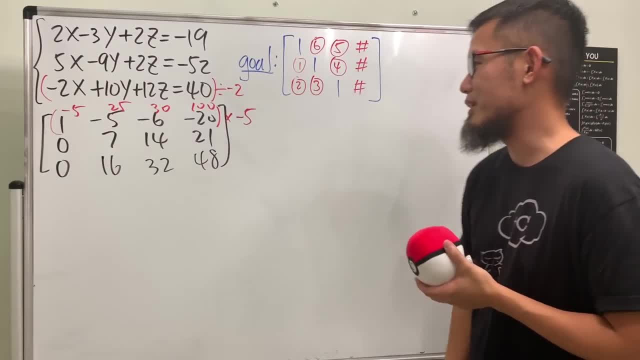 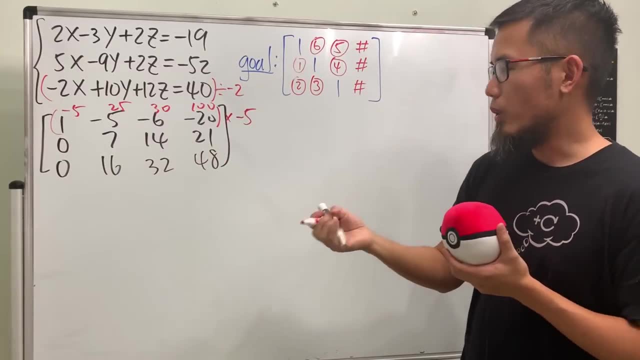 and then just do that to yeah to your teacher, I guess. Okay, So we got the first column done. Now I want to make this, right here, equal to 1.. Well, right here we have 7,, 14, and 21,. 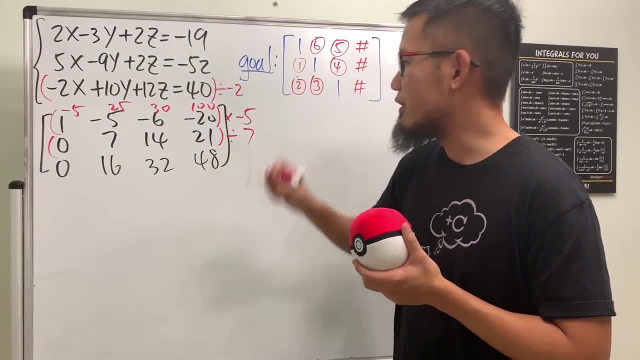 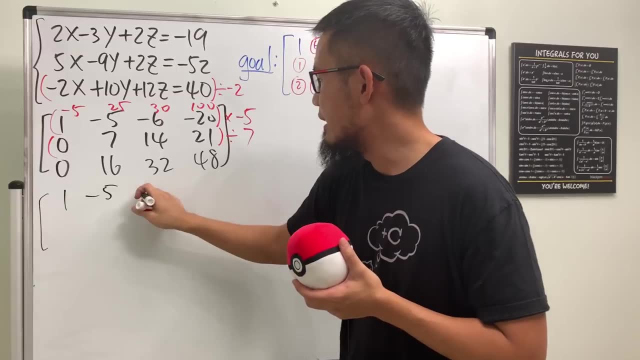 which is very nice, because we can just divide everybody by 7 here and no fractions. huh, Pretty good. Okay, so the first row stays. We have 1, negative 5, negative 6, negative 20, and then we get 0,. 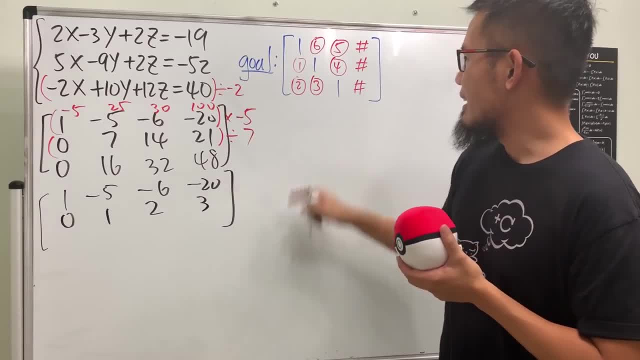 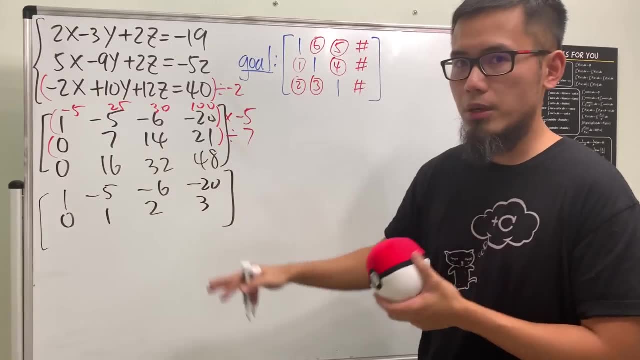 1,, 2, 3.. Perfect, Okay. Now I want to make this right here equal to 0.. This is 16. And what we can do is just multiply everybody right here by negative 16.. So let's do that. 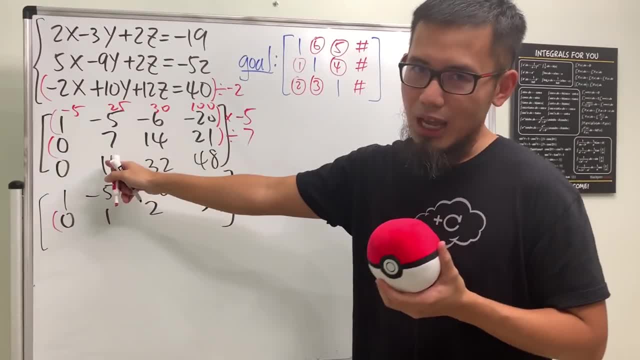 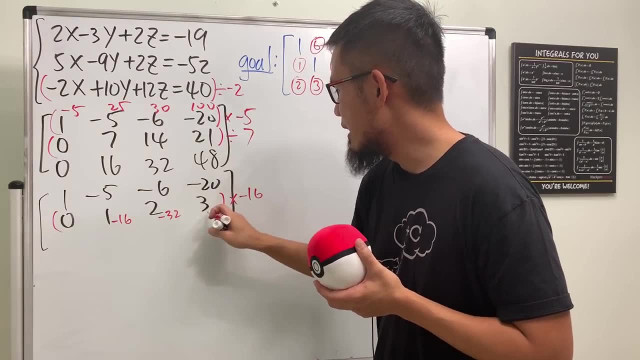 Multiply this by negative 16.. Or, if you would like, you can actually divide everybody by 16 here and then yeah. Anyway, though you see, this is negative 16,, negative 32, and then negative 48. Combine to them. 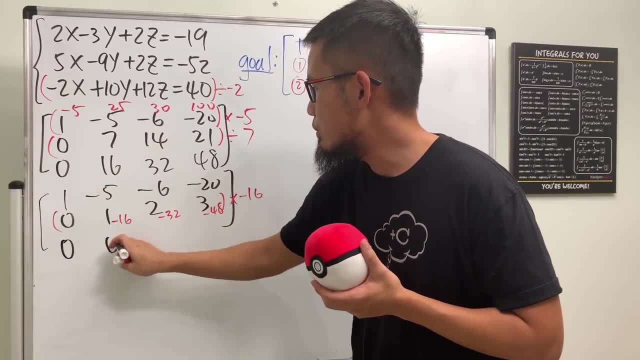 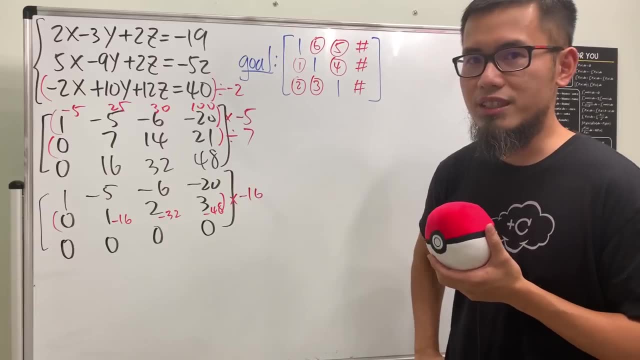 and then you see we get 0, and then 0, and then 0, and then 0.. Very interesting. Now, in this situation, unfortunately there's no way for us to end up with 1, 1,. 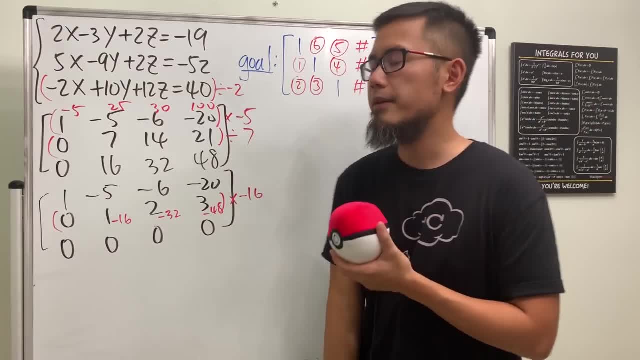 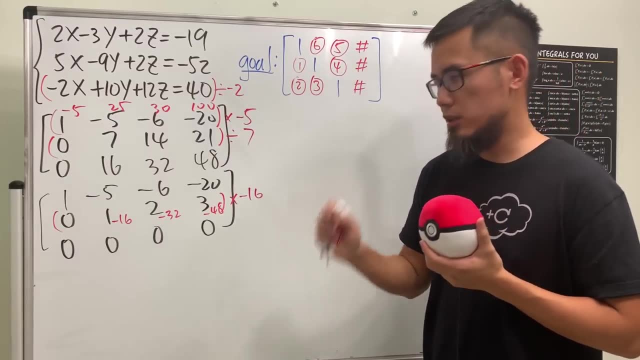 1 right here, because the last row is just all 0s right. So here is the different scenario compared to the first example. We actually will have infinitely many students And well, I cannot get rid of these two numbers anymore. 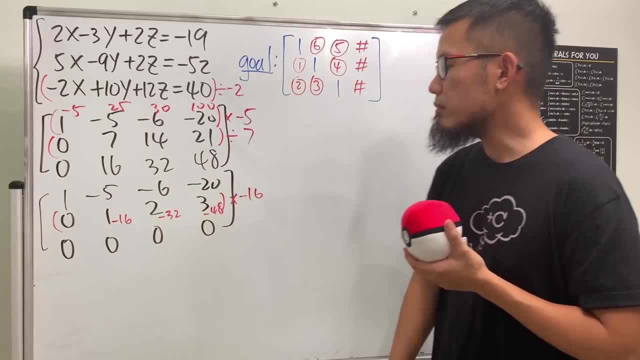 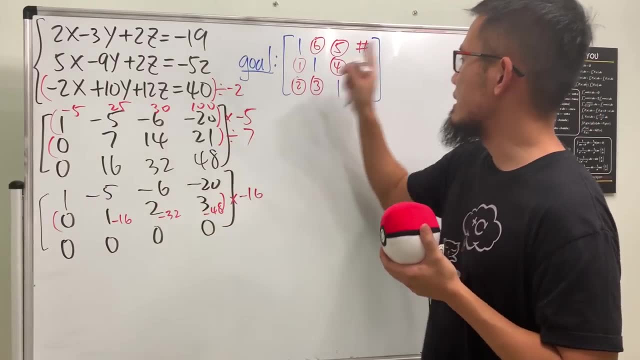 because I don't have any number in this entry. right, And you can also use some technical terms. We do not have a pivot in every row, But whatever, Oh man, but I think we can still make this equal to 0.. 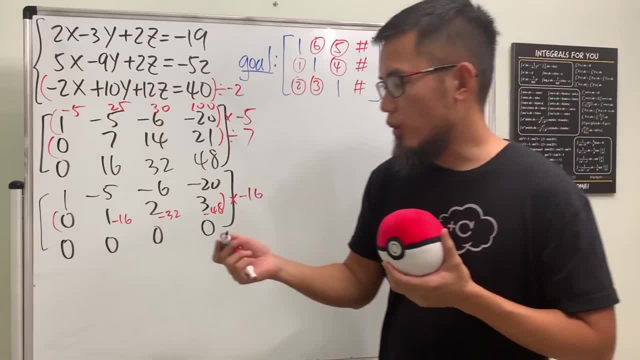 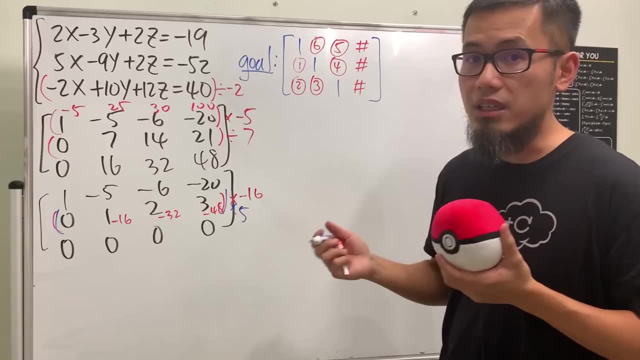 So let's go ahead and do that. To do so, I will multiply this row by negative. well, by this is negative 5 already, So 5 is enough. So we get 5,, 10, and then 15.. 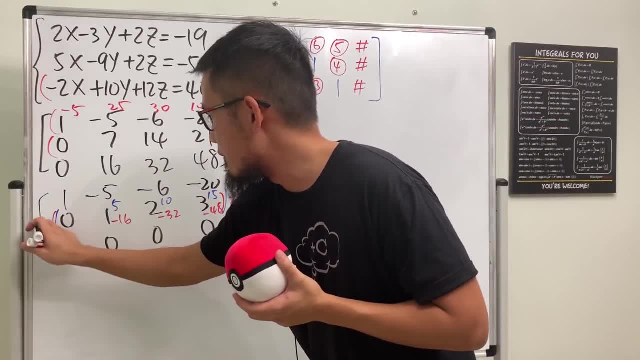 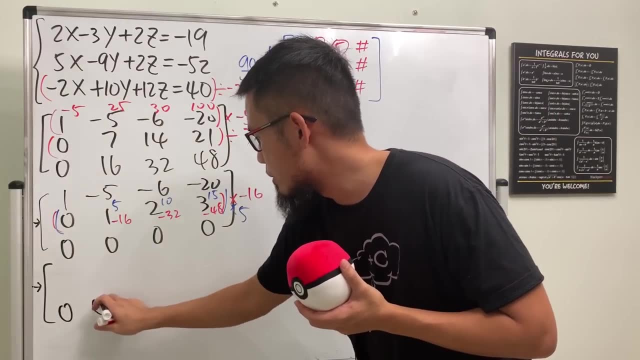 So, ladies and gentlemen, for this right here I've got a little arrow, So let's see. Well, in the end we see that we will just get 0, 0,, 0,, 0, and then 0,. 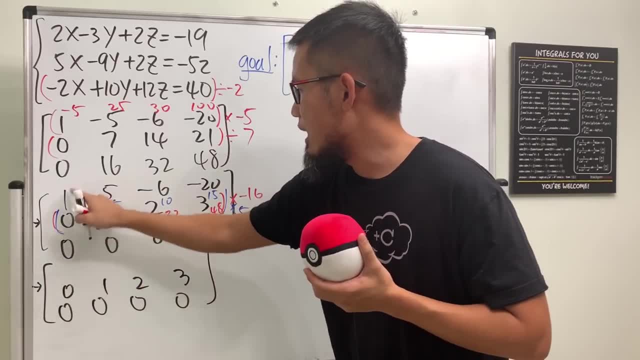 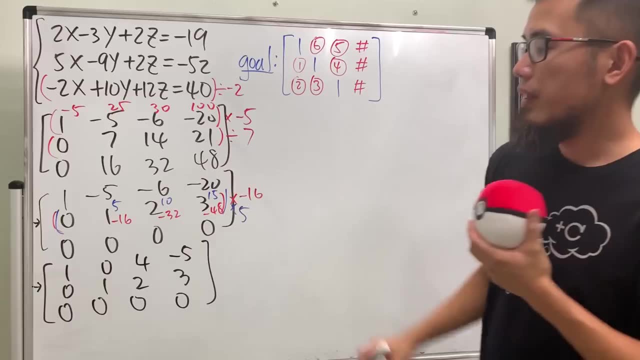 1,, 2,, 3,, which is pretty nice, And lastly, this becomes 1,, 5 and that is 0,, this and that is 4, and this and that is negative 5.. So that's pretty much the final product that we have. 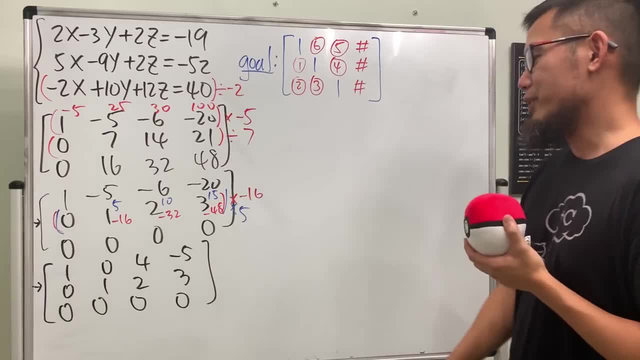 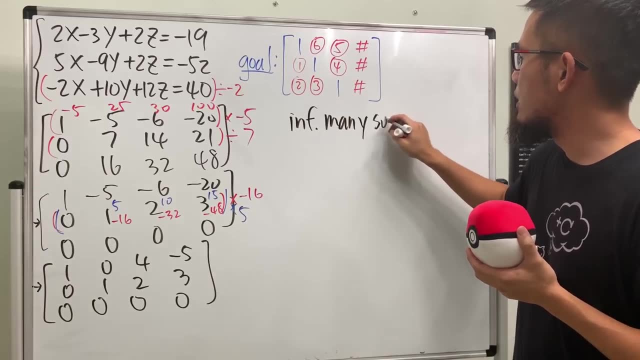 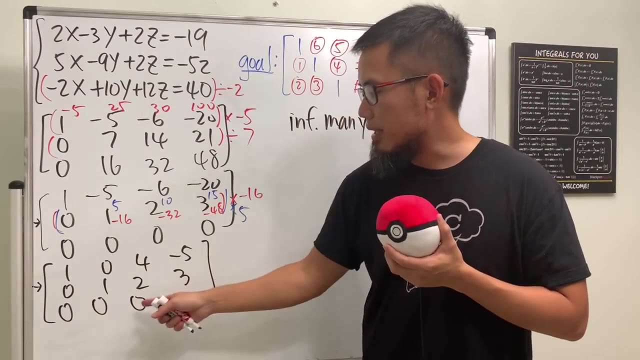 Not like multiplication, but like final result that we have. Okay. So how are we going to interpret that? Well, we have infinitely many solutions. Alright, Whenever you have 0, 0,, 0, 0, you can just imagine, you have 0x plus 0y plus 0c is equal to 0. 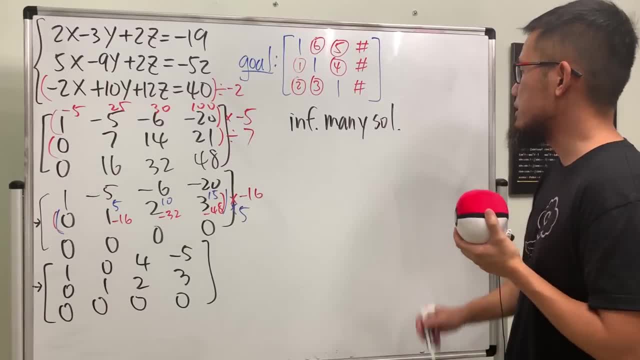 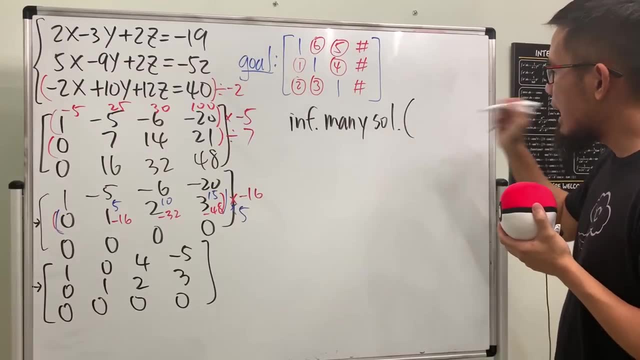 And, as you can see, that's always true. You have infinitely many solutions for this And in this particular case, the intersections of all these three planes is a line, So I will just write this down right here for you guys: The intersection. 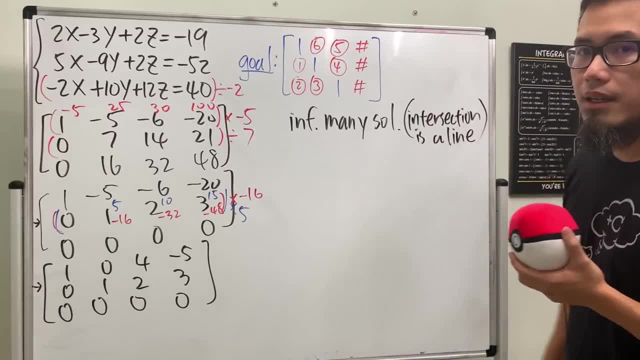 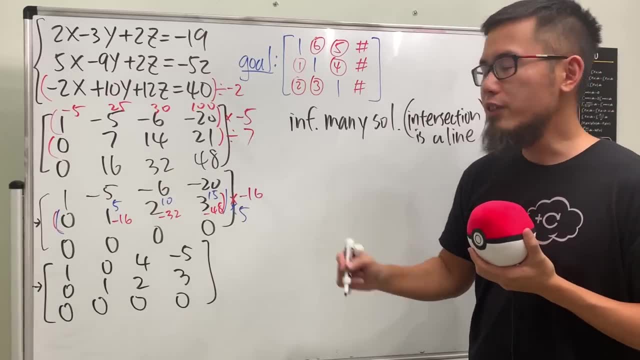 is a line. This is another situation, though, but that will be later on. Okay, So we have this and that, In this case, we do have one free variable, So I will just write this down right here for you guys. 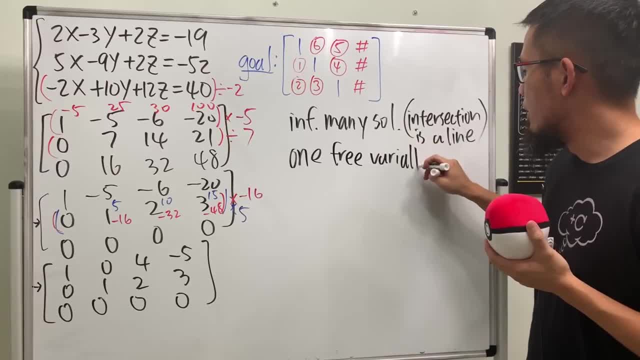 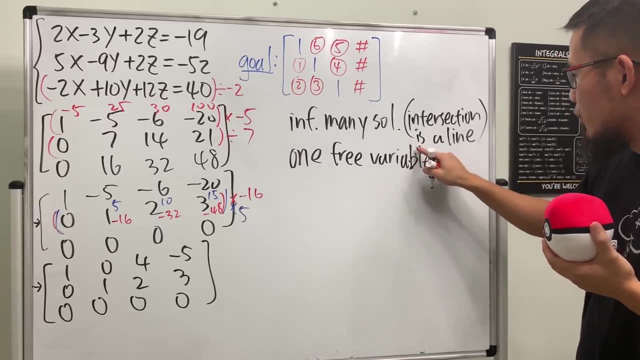 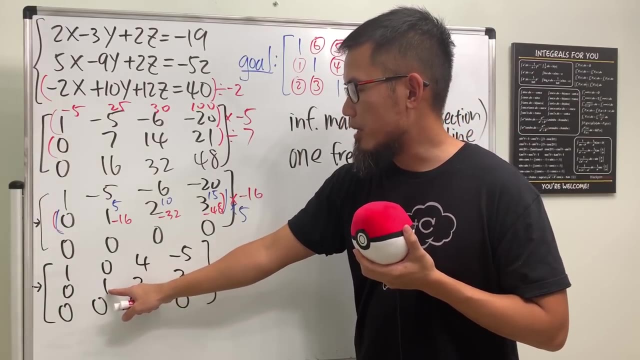 One free variable. So you can see a bo, a bo, Yeah, One free variable and the variable will be z. We'll just use z right here for the free variable, Because you can read this right here as y, 1y plus 2z equals 3.. 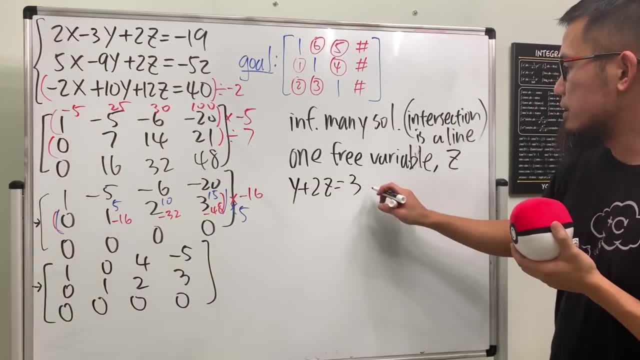 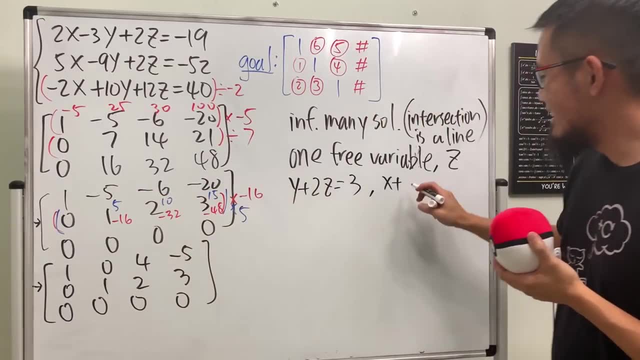 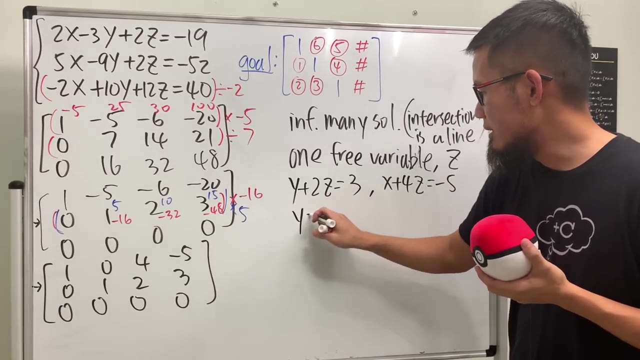 Similarly, you can also read the first row as x plus no y. That's why we want to get rid of that right here earlier. This right here is 4z and we have negative 5.. Well, move this here we get. y is equal to negative 2z plus 3.. 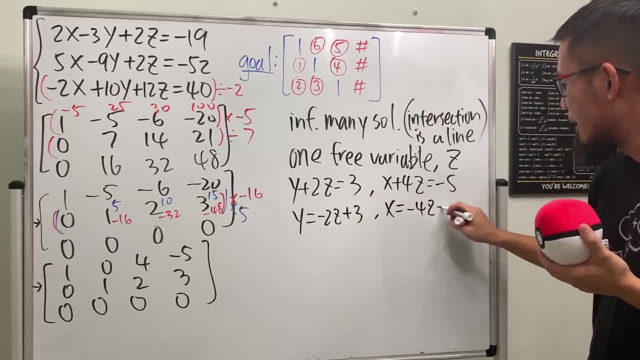 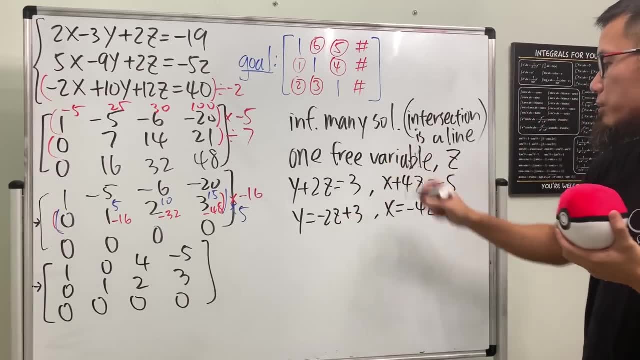 And likewise we get: x is equal to negative 4z minus 5.. As you can see, x and y, they are based on z, So z is the free variable, named whatever you want. All right, And this is how you can write down your answer. 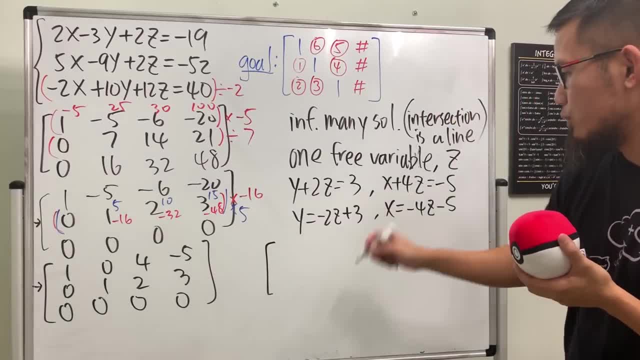 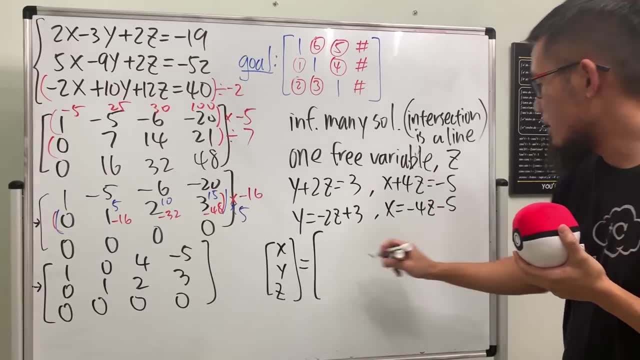 You can write it as a solution set just by putting down the set notation. But I will just write this down for you guys: x, y, z. Well, what's x, x is that? So we have negative 4z minus 5.. 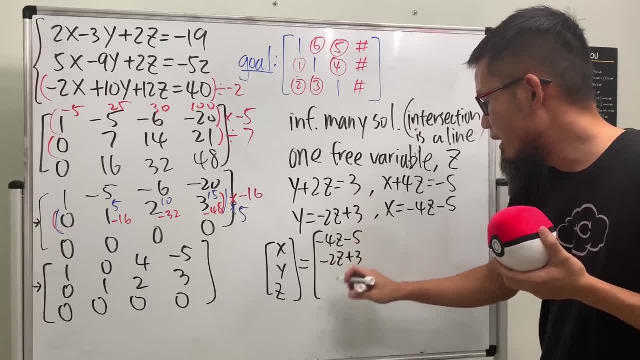 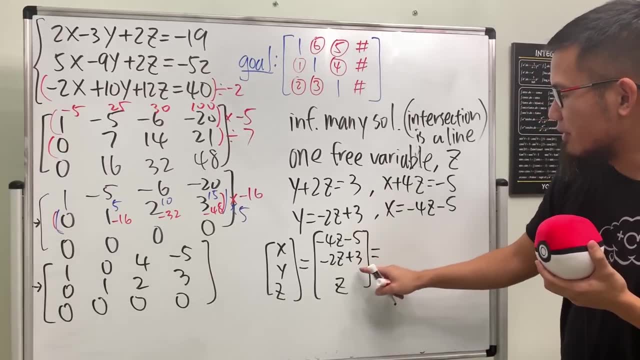 And then y, is that Negative 2z plus 3.. And what's z? z is just z, Just like that. Okay, Now I'm going to write down the constant first, So I will put down negative 5,. 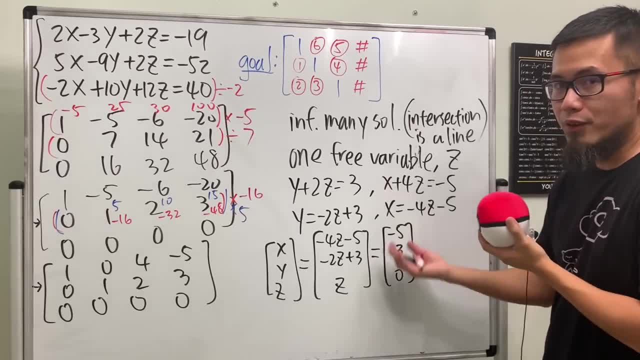 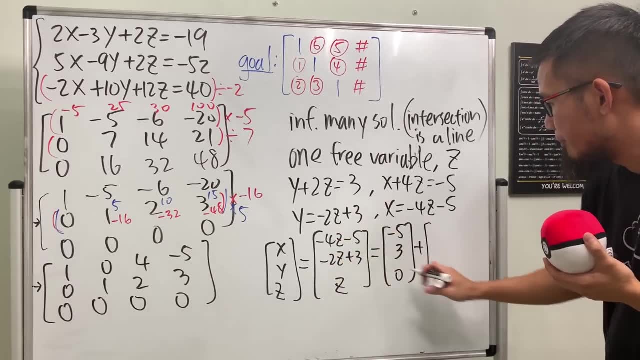 3, and 0. So this is going to be my first factor, And then I'm going to put down second factor. Then they all have the z, But I will write down the coefficients though, So I will just add. 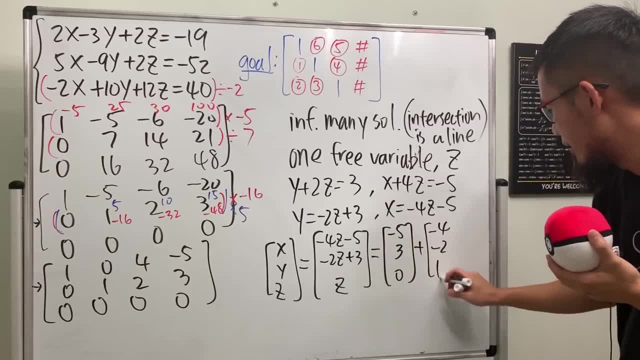 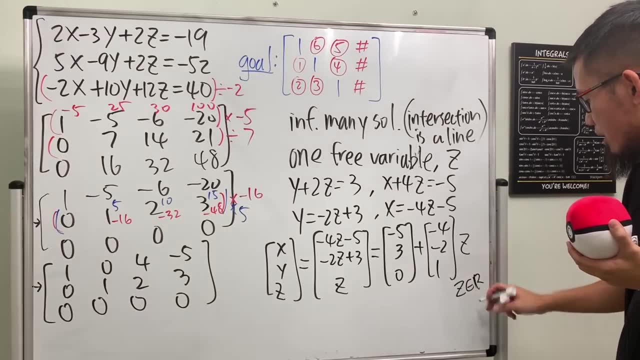 This is negative 4,, negative 2, and 1.. And then don't forget to multiply by z, Like this, And you can also just say z is a real number. Yeah, depends, But I think this is clear enough. 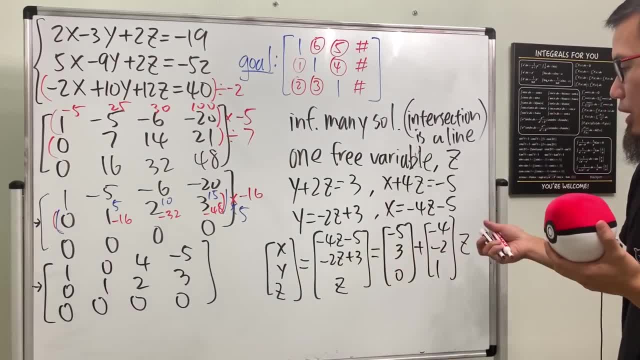 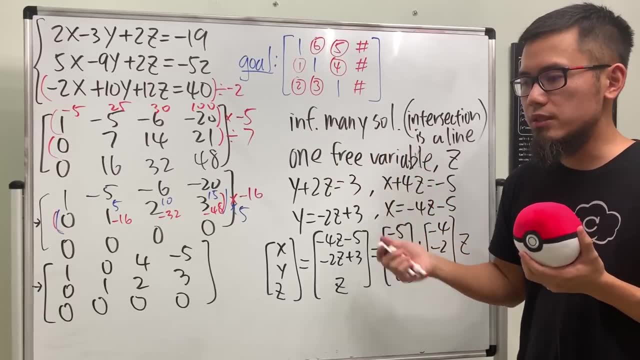 Right, If you don't put it in the set-button notation, the set notation, I don't think you have to do that. That's pretty much it. And notice that because we have infinitely many solutions, that means we do have a solution. 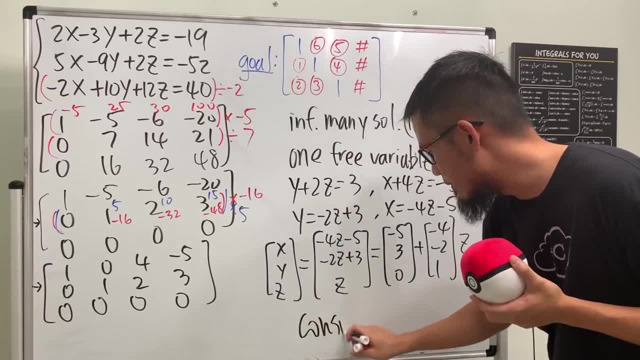 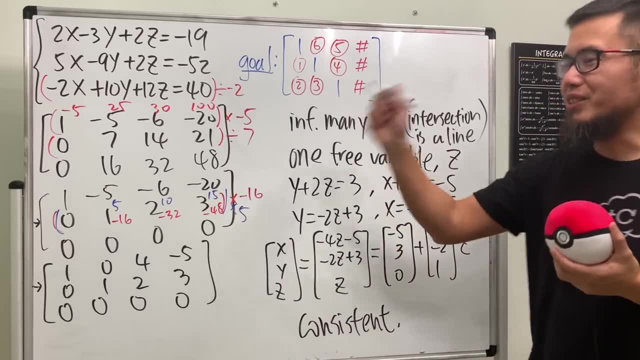 So this system right here is consistent, Right, But that's how you wrote reduce And these are the interpretations for that result. Now let's look at the third example. Okay, are you guys ready to write reduce? I don't know. 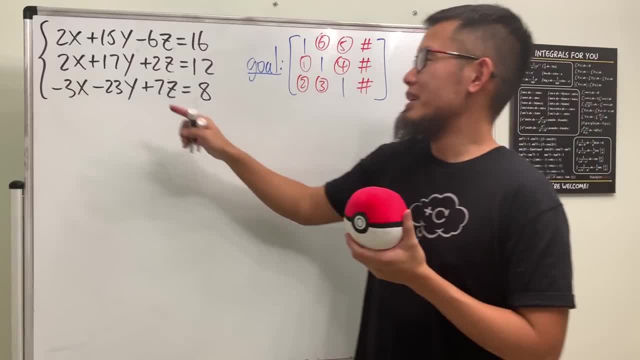 but here we go. So if you look at all this right here, unfortunately we cannot avoid fractions, So I'm just going to take the first equation as how it is, And then I will just divide it by 2. And that will give me the 1 right there. 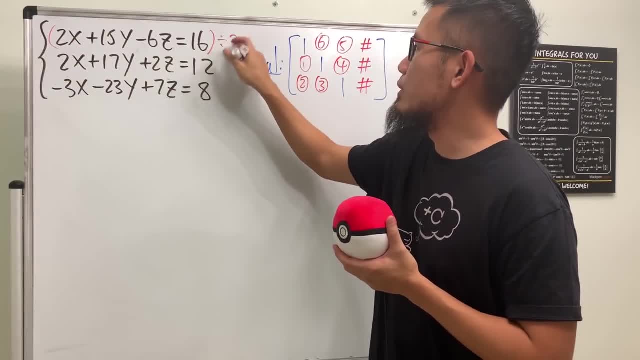 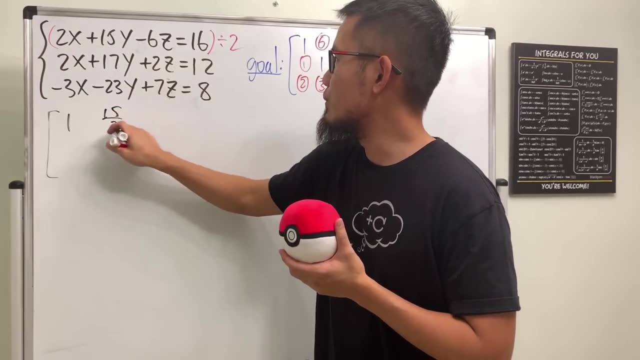 Right, So here we go. First we will have 1., And this is 15 over 2.. And then we get negative 3. And then 8.. So that's our first row, And then I want to make sure that. 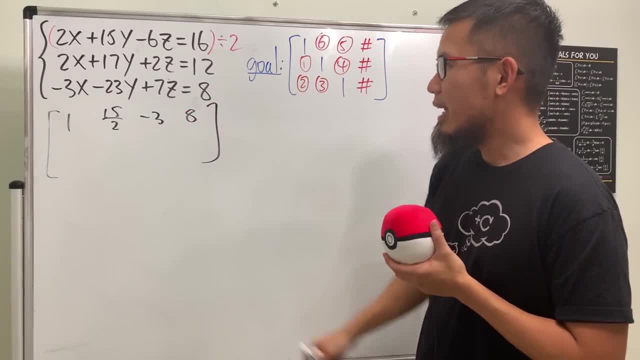 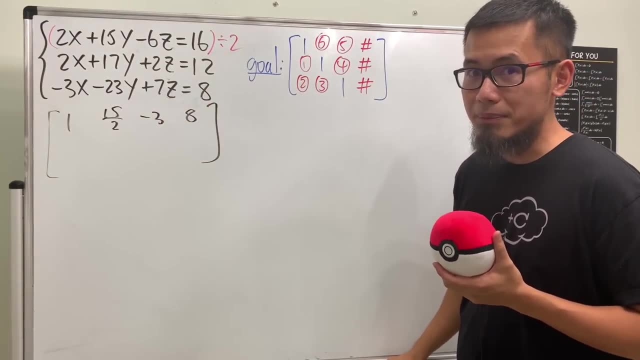 the first row is equal to 1.. So I'm going to write this down And then I want to make this right here, equal to 0. What we can do is just look at the original equation right here And then we will multiply everybody by negative 1.. 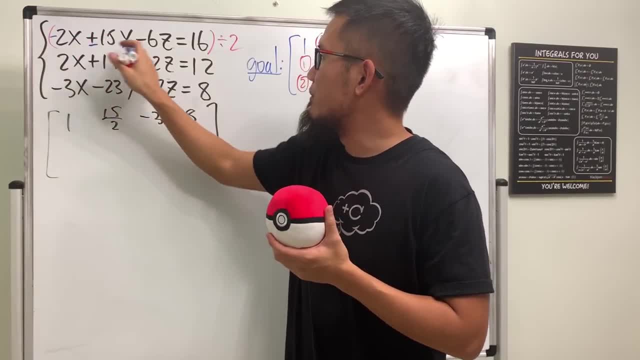 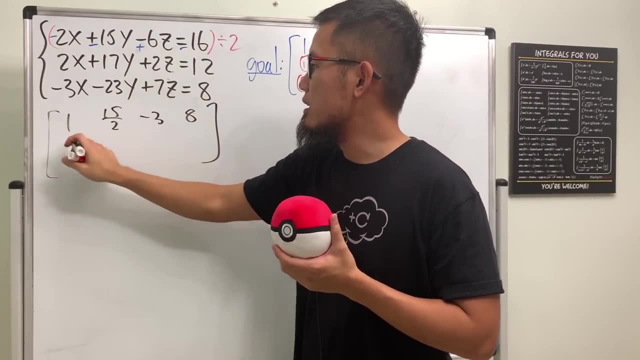 And when we do that, we can look at this as negative 2, negative 15, positive 6, and negative 16. And then just combine them So we get this and that together is 0. This and that together is 2.. 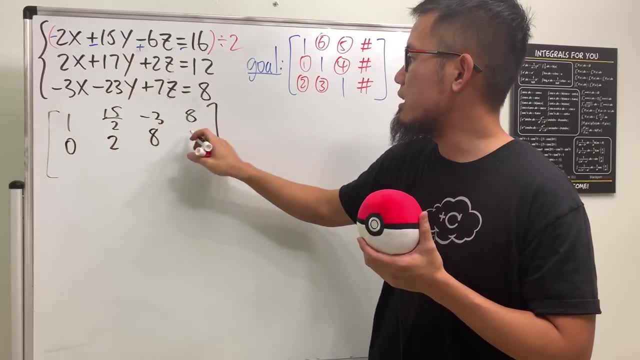 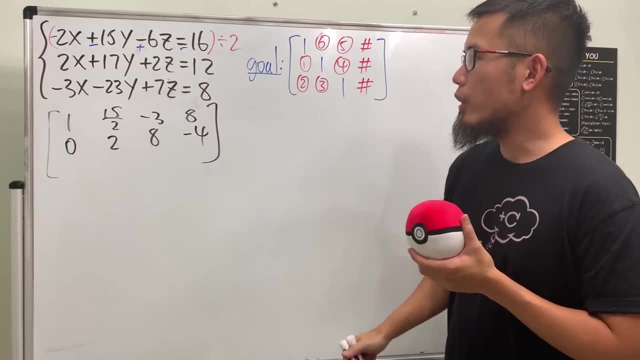 This and that together is 8.. And this and that together is negative 4.. Alright, Now, if we make this equal to 0,, well, I will take this row right here, multiply it by positive 3, and add it to there. 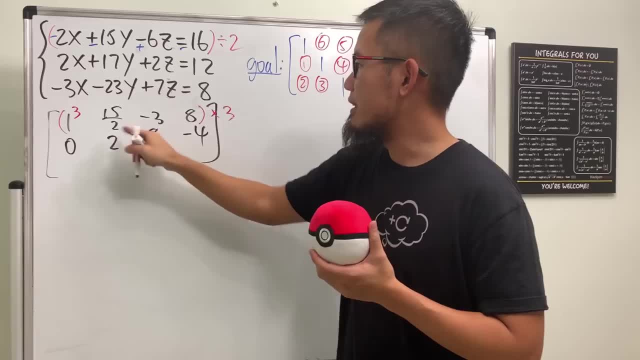 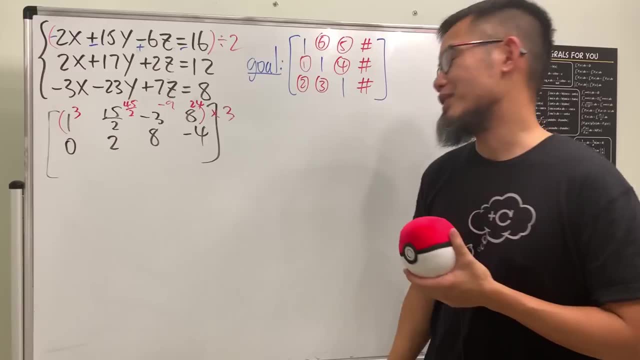 So multiply this by positive 3, we get 3.. This and that is 45 over 2.. And this and that is negative 9.. And then 24.. 8 and 24.. Kobe Bryant, of course. 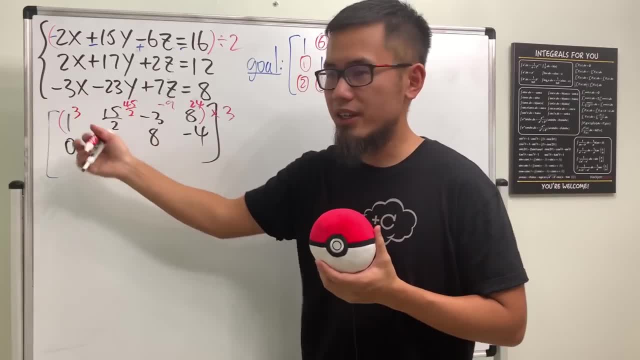 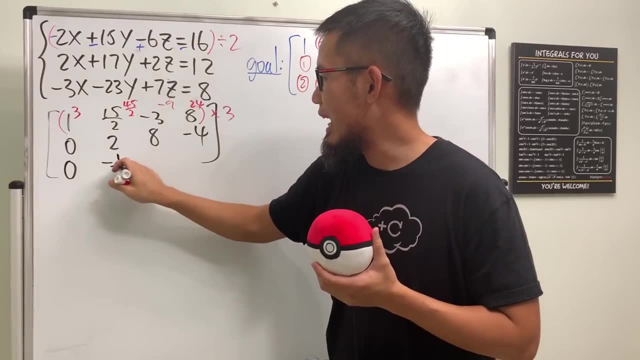 Rest in peace, of course. Alright, This and that together we get 0. And this and that together this is the same as negative 46 over 2. And that so we get negative 1, half This and that. 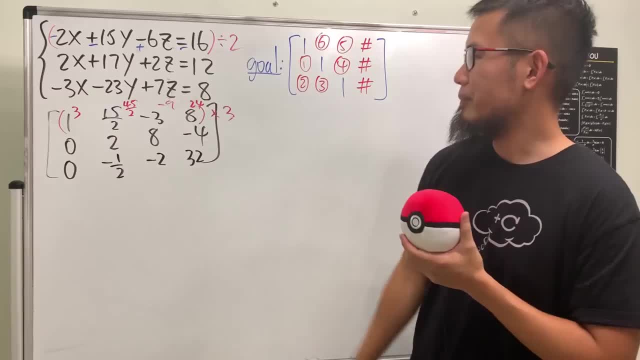 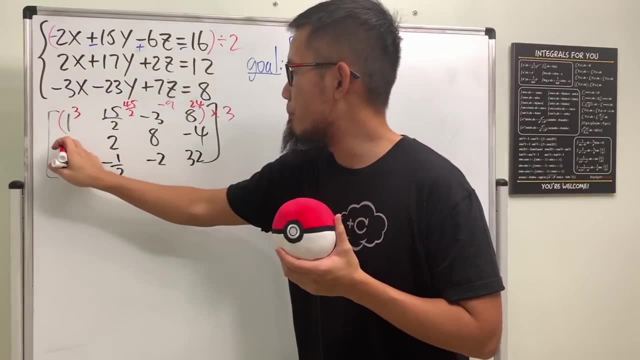 we get negative 2.. This and that we get 32.. Okay, So we got the first column done. Now we need to make this right here: equal to 1. And we can just do so by dividing the second row by 2.. 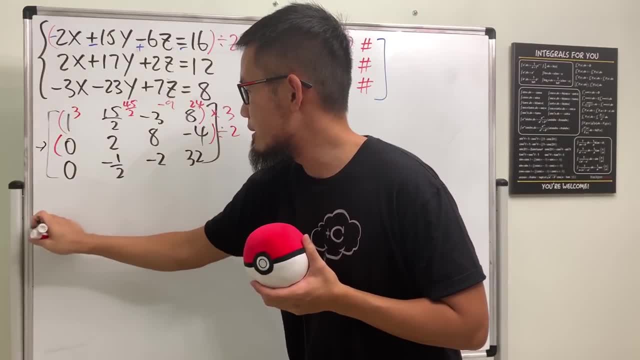 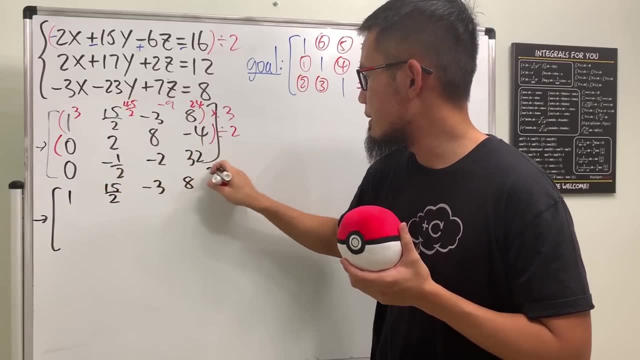 So have a look. This becomes- we'll draw the arrows. The first row stays 1, 15 over 2, and then negative 3, and then 8.. But the second row becomes 0, 1,. 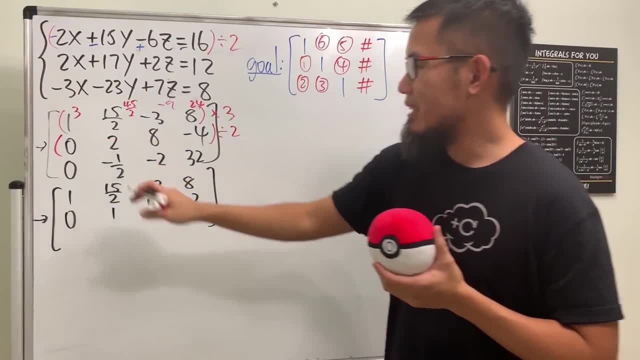 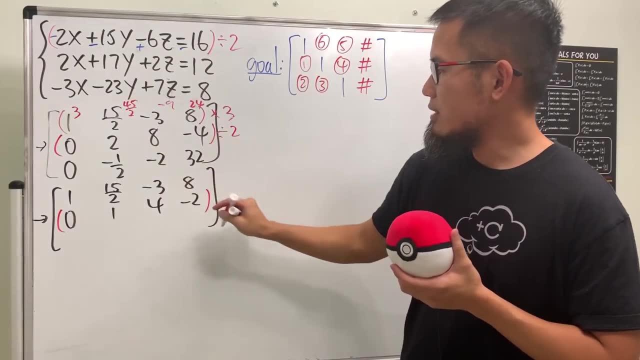 4, and negative 2.. And lastly, we want to make this right here equal to 0, right, And we will actually multiply this by positive 1 half. So now you see, we get positive 1 half here. 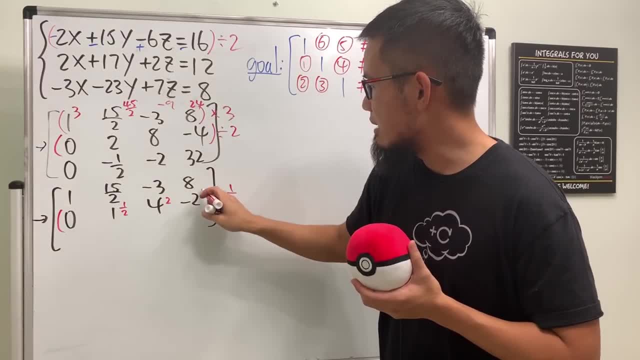 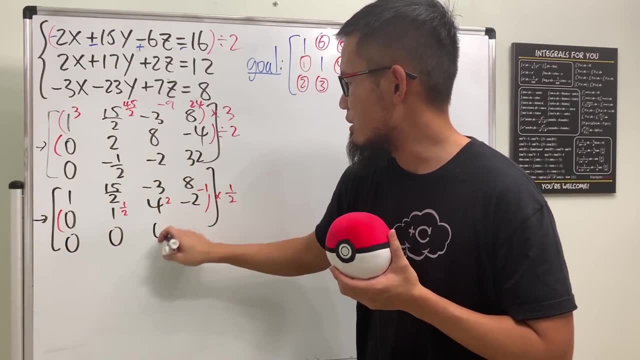 And this ta-da is going to be 2.. And this and that is negative 1.. Alright, This and that together, we get 0.. And this and that together, we get 0.. Negative 1 and 32 together. 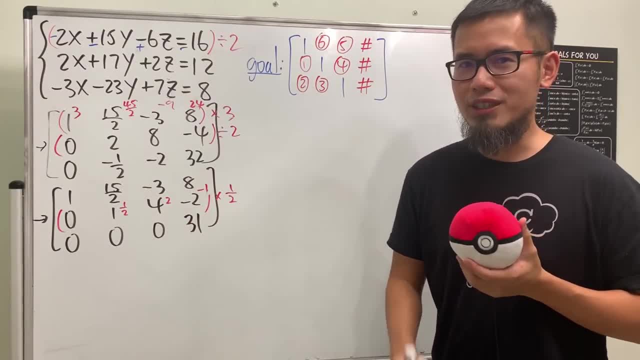 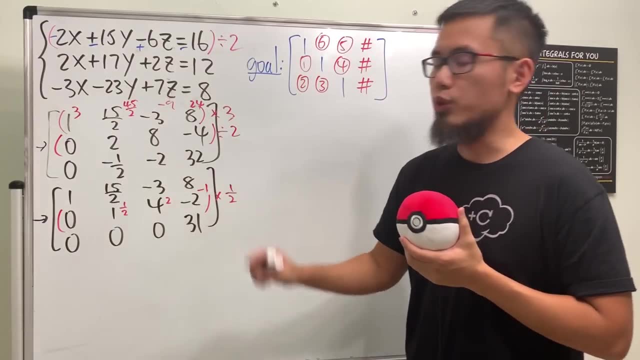 we get 31.. Hmm, another strange situation. huh, 0, 0,, 0, 31.. In another word, 0x plus 0y plus 0c is equal to 31.. It is not even possible. 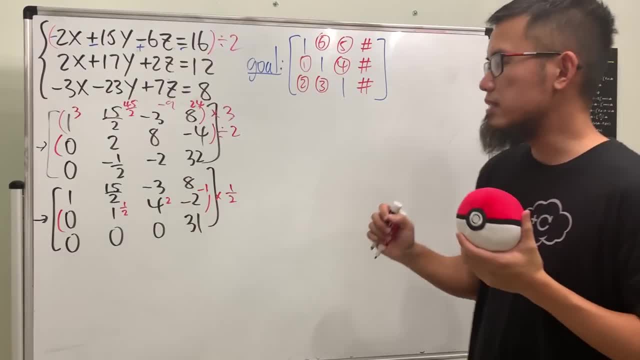 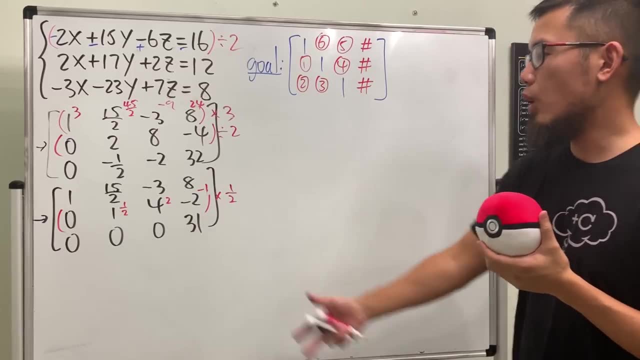 No, So this right here is actually an inconsistent system And we actually do not have any solutions for this And you can actually kind of just answer it, but you can also just keep on going, depending on your instruction. I will say: Let us see how we can keep reduce the fraction. 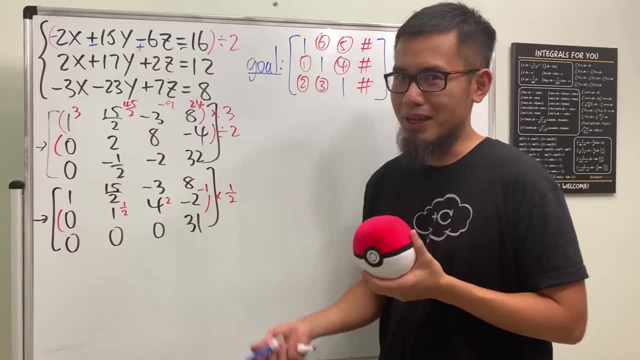 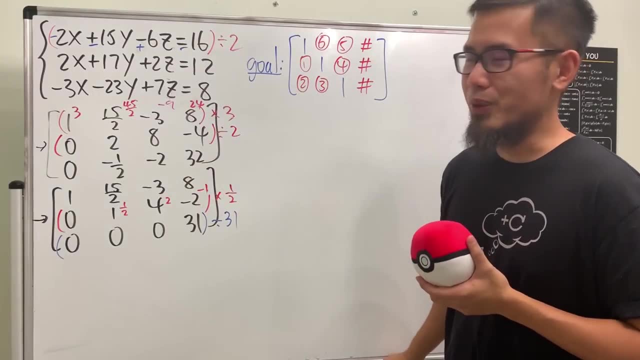 One of the things that you can do is divide this by 31.. So you can make this equal to 1.. That's pretty much what we can do right here. It's kind of cool, right? So let's see, I am just going to write this down here for you guys. 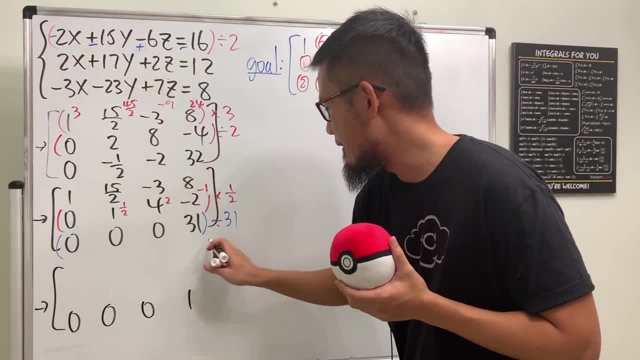 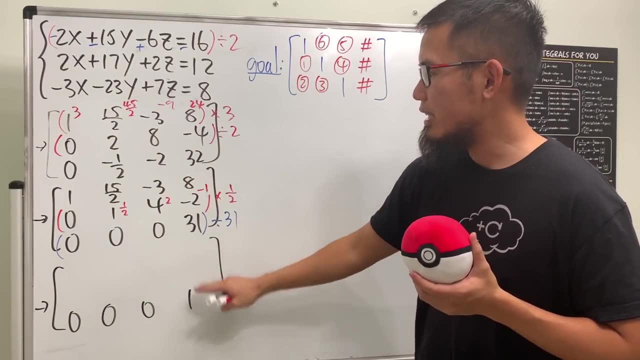 We get 0,, 0, 0, and then 1.. Alright, Now what I will do is I will multiply this by positive 2 and then add it to the second row. Alright, So I will add this to the second row right here. 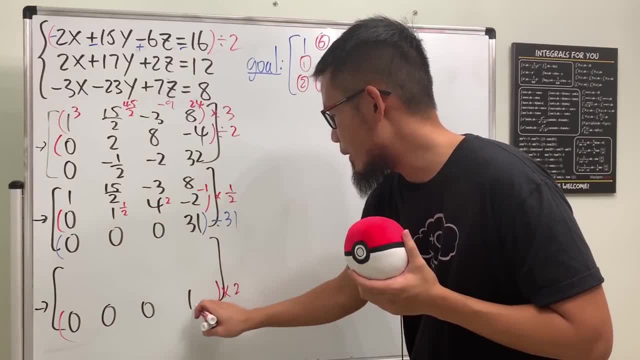 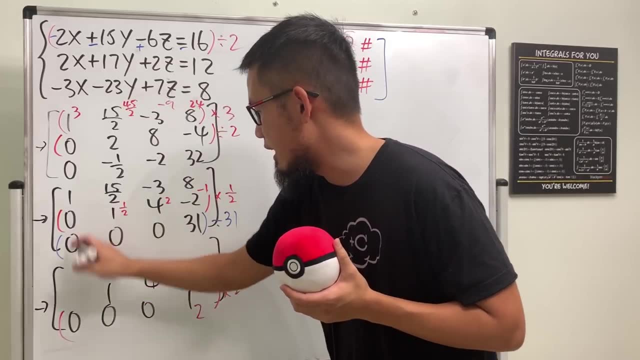 So I will multiply this by positive 2. And now that will just give me a 2.. So 2 plus that is just going to be 0. And then the 4 stays, And then this 1 also stays, And likewise this 0 also stays. 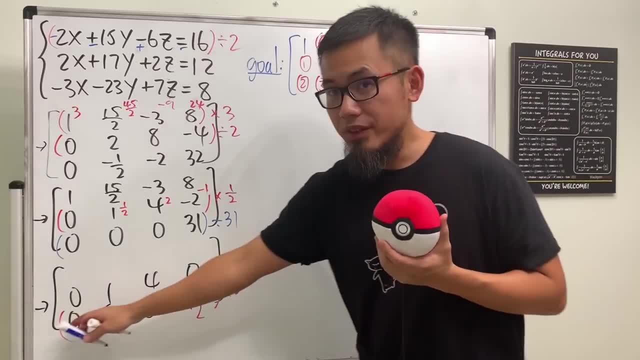 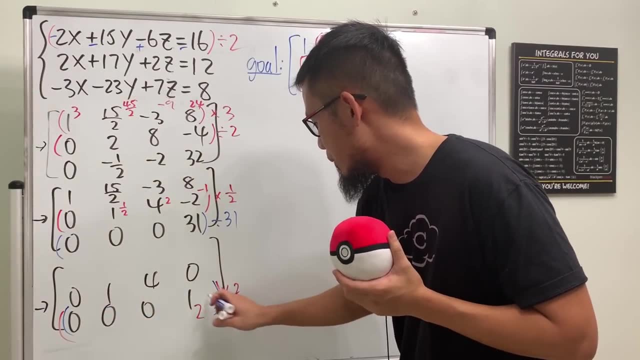 And I will multiply this by negative 8 and then add it to the first row. So multiply this by negative 8.. I will end up with negative 8 right here, Plus that We get 0. And then the rest stays right. 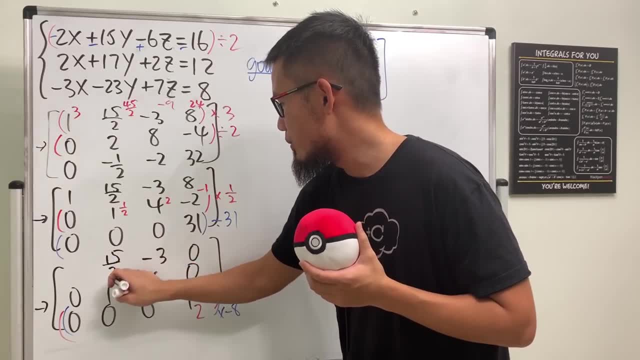 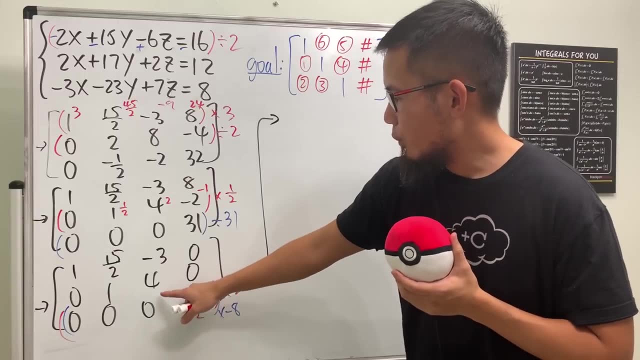 So we get negative 3,, 15 over 2, and then 1.. Like that, Hmm, What else can we do? Well, there is no way for me to make this equal to 0.. Likewise not, But we can make this equal to 0. 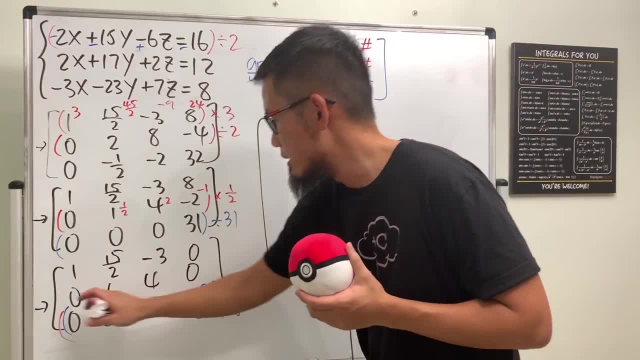 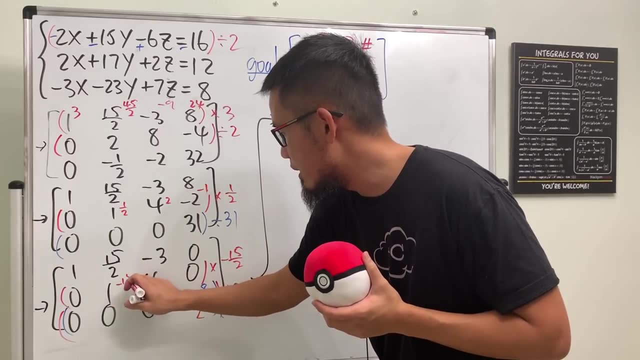 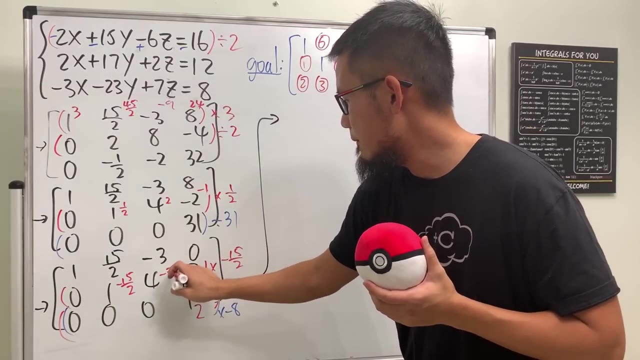 And what we can do is just multiply this row by negative 15 over 2.. And we get negative 15 over 2.. And this and that, Of course, you get the 2 reduced, which is going to be negative 30.. 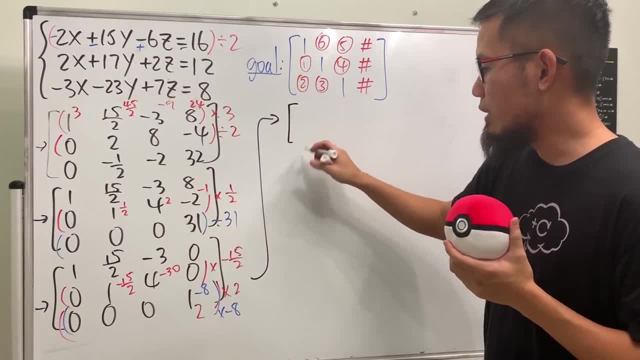 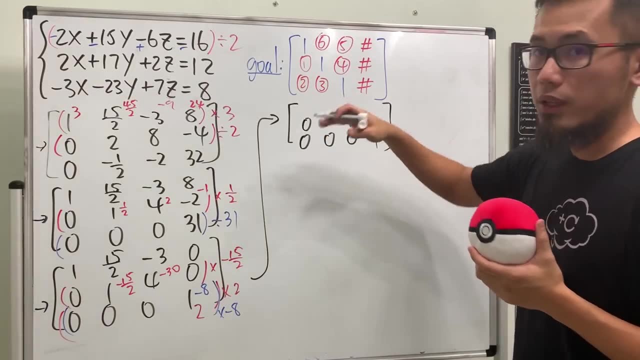 All right. So let's see. The final result that we have is 0, 0, 0, 1.. And then 0, 1, 4, 0. And for the first row, this and that is 0.. 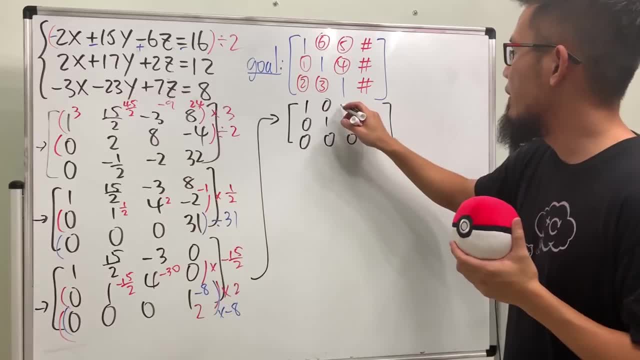 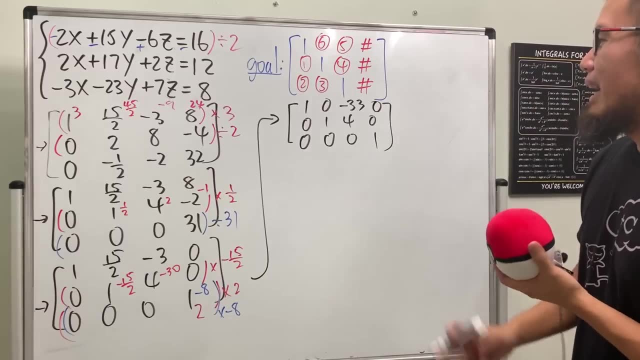 The 1 in front And then 0. This and that is negative 33. And lastly, we have that 0. So that's the final result, right, But anyway, 0,, 0,, 0, 1.. 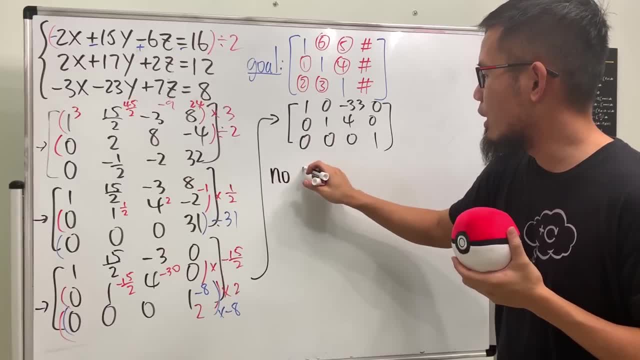 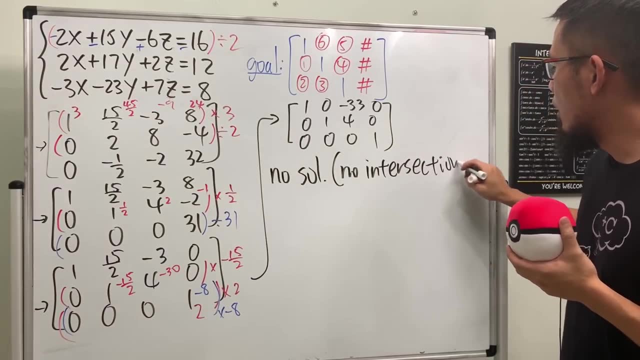 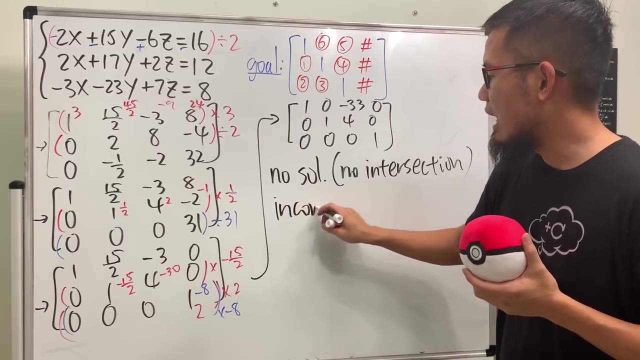 This right here tells us that this right here has no solutions And there's actually no point of intersection of these three planes. And again, when you don't have any solutions, this system is what we call the inconsistent Right. So that's it. 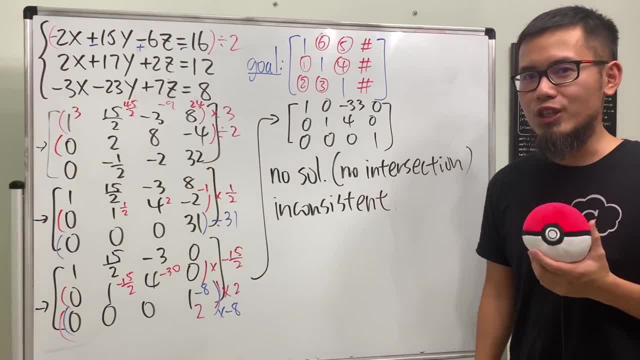 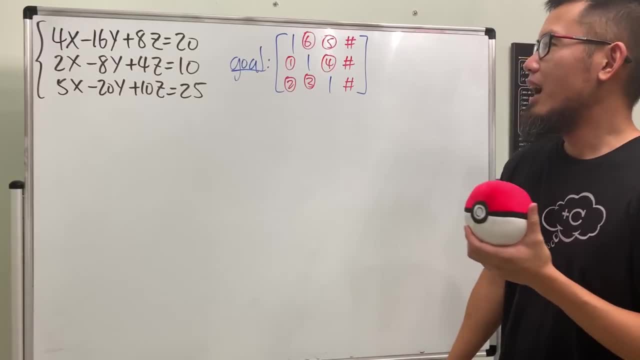 Again, just know this situation. And there's one more situation that we have to go over. Have a look right here. Okay, So let's see what's so strange about this system of equations. Again, we want to make this right here: equal to 1.. 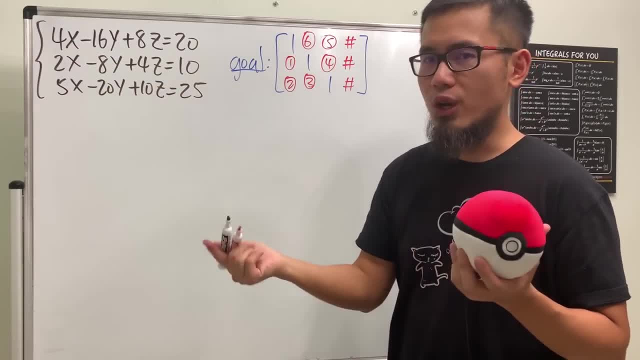 And it seems like we can just divide the first equation by 4.. So let's go ahead and do that, And we don't end up with fractions, So I am not worried about it at all. right, So divide everybody by 4.. 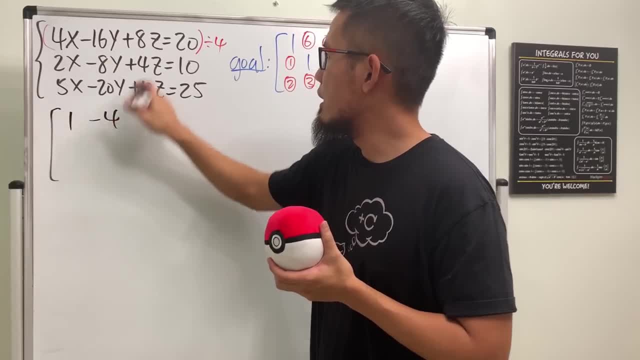 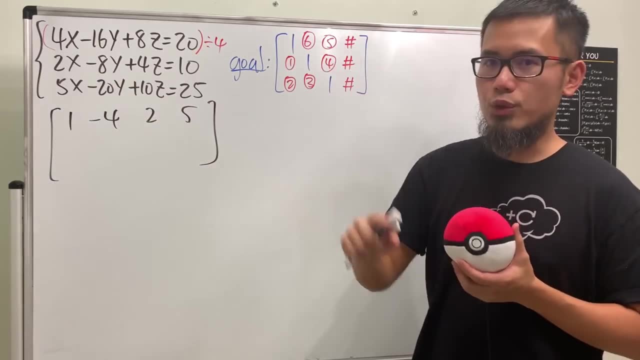 And we start with 1, negative 4, and then 2, and then this is 5.. Okay, Now we need to make this equal to 0, and here we have 2 already. So what we can do is: 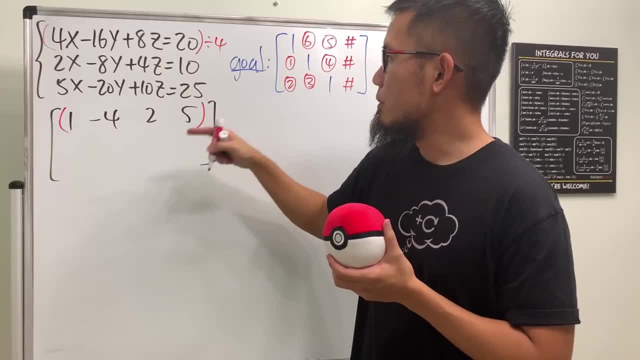 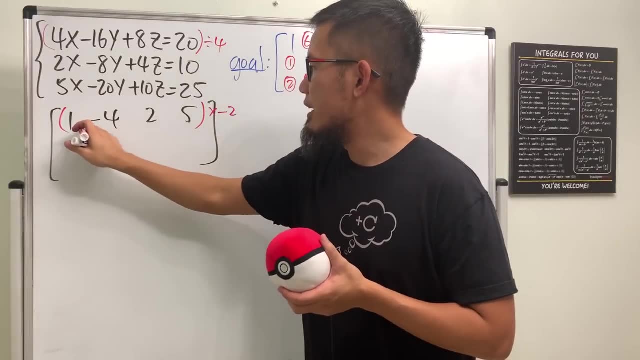 you can multiply everybody right here by negative 2.. Or you can just divide the first equation by negative 2.. Up to you. I will multiply everybody right here by negative 2.. We get negative 2,, positive 8,, negative 4, and then negative 10.. 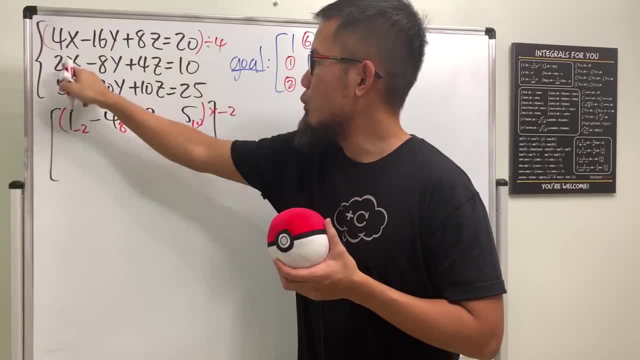 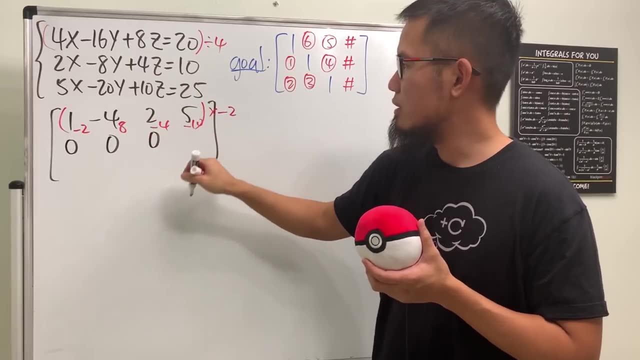 And I will take these numbers combine right here. I will get 0, and then 0, and then 0, and then 0. Seriously, Maybe just bad luck, I don't know. All right Now, we want to make this right here. 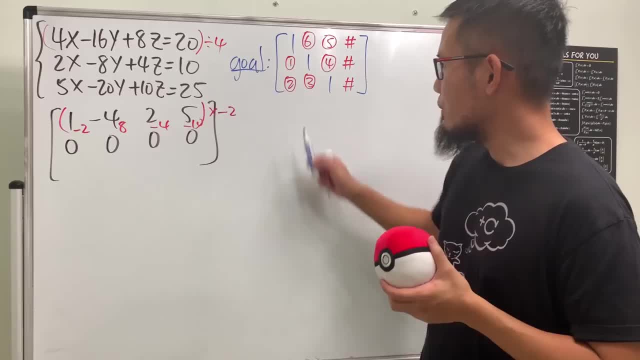 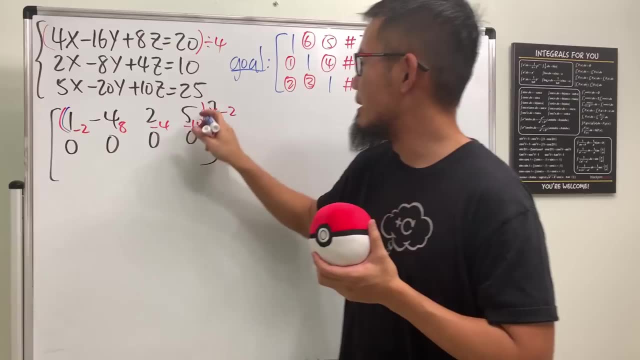 equal to 0.. Okay, That's 5.. So I am going to multiply this by negative 5.. And when we do that, we will end up with negative 5,, positive 20,, negative 10, and then, lastly, 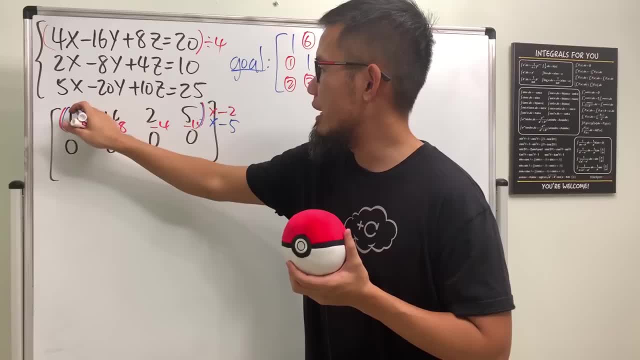 we have the negative 25.. But if we combine this and that, we end up with negative 5,, positive 20,, negative 10, and then, lastly, we have the negative 25.. But if we combine this and that, 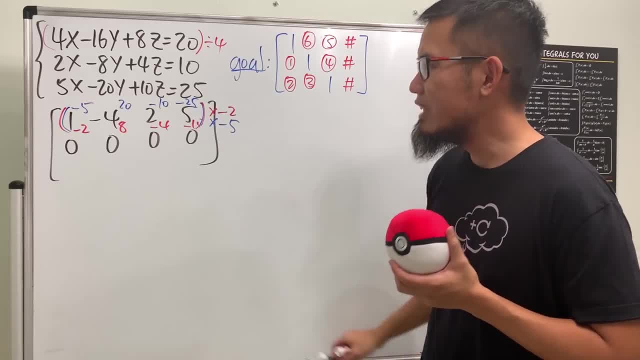 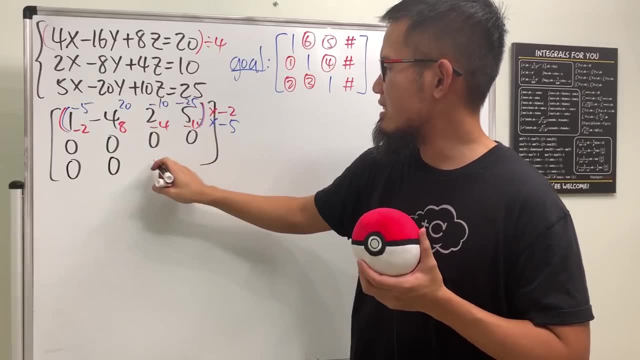 we end up with negative 5,, positive 20, negative 10, we combine this and that, yes, we have the 0 that we want. but this and that together is 0,. this and that is 0, and then this, right here: 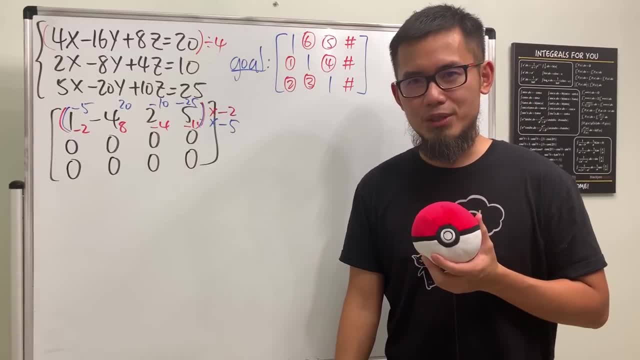 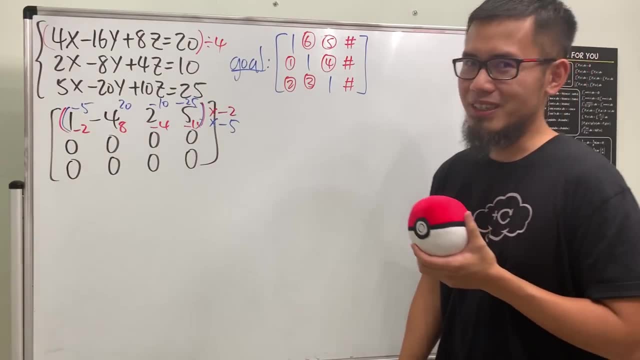 oh, my god, it's just all 0s. The truth is, in fact, they are pretty much all multiples of each other, constant multiples of each other, And in this case, we are pretty much done in terms of reducing the matrix. 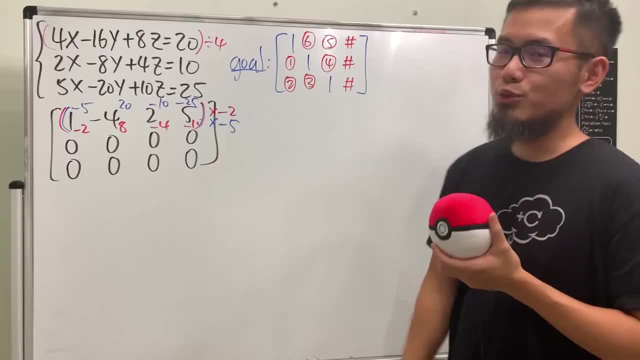 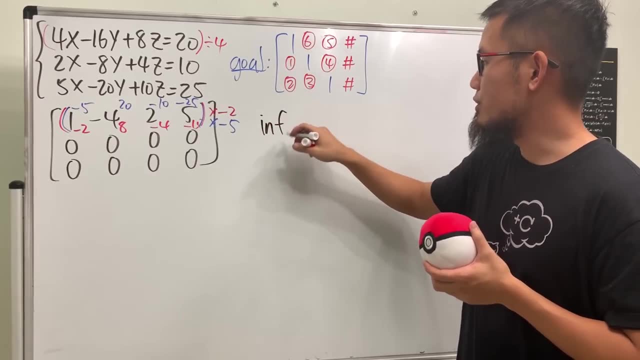 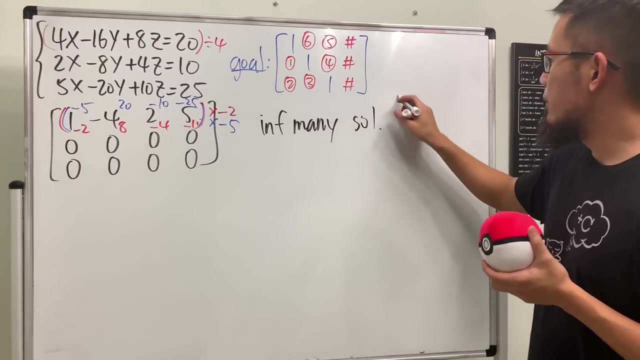 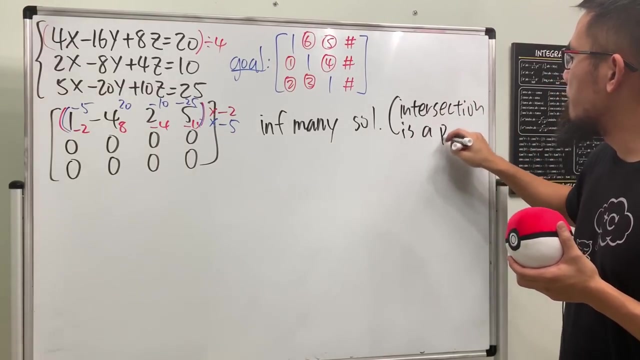 And here we go. How many solutions do we have? You see, we have a row of 0s and then we have infinitely many solutions. But in this case, the intersection, the point of intersection, is a plane instead of a line. 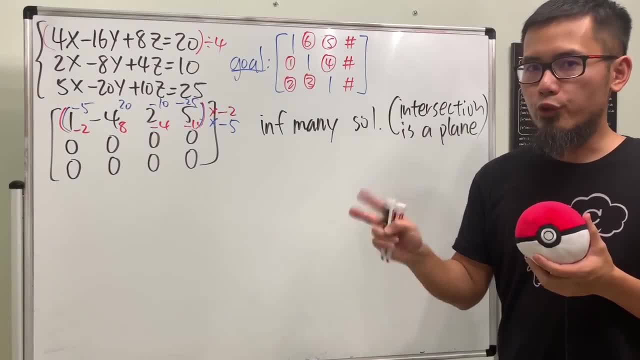 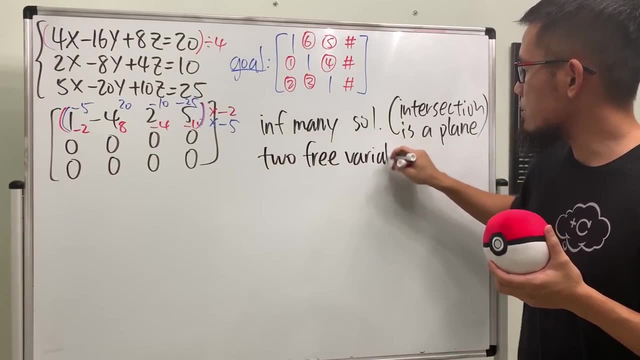 Because in this particular case we actually have two free variables. So let me just write this down right here for you guys: Two free variables, And I'm just going to use y and z. Have a look of the first row right here. 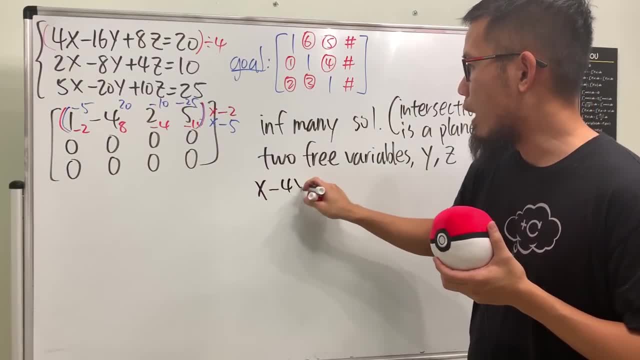 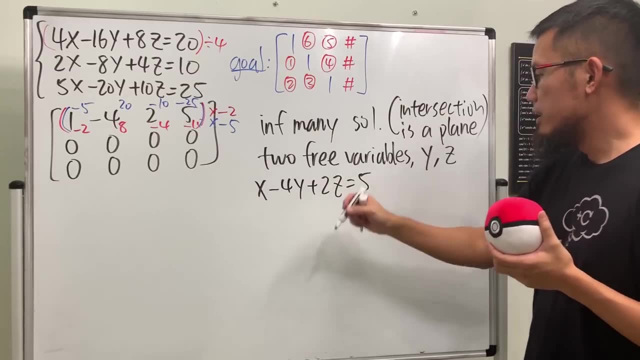 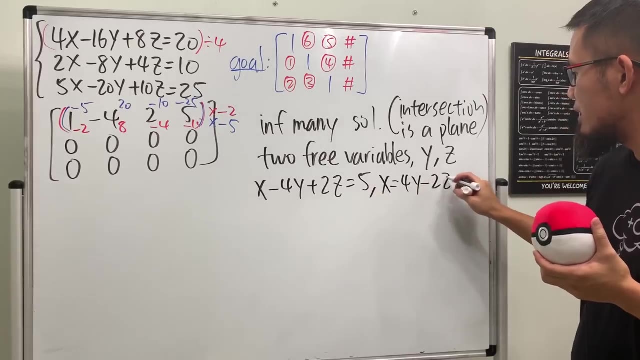 We can read this as: 1x minus 4y plus 2z is equal to 5.. And I'm just going to kick this to the other side. This is telling us that x is equal to 4y minus 2z. 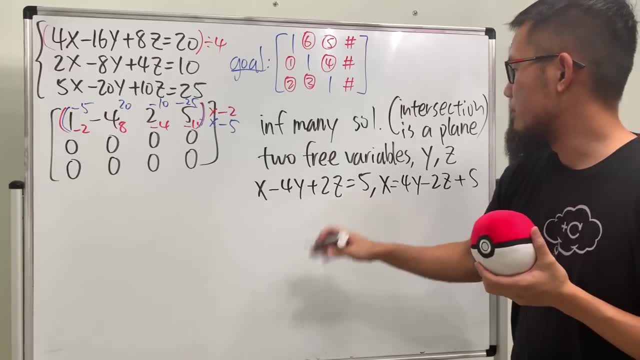 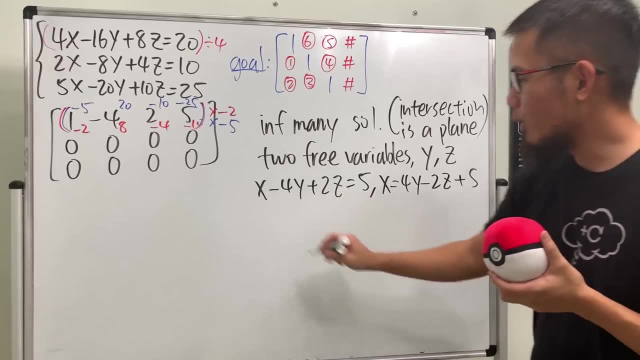 and then plus 5.. And then x and y are free, Right? So you can see. x, I mean y and z- are free And x is based on y and z. And now, if you want to write your solution: x, y, z. 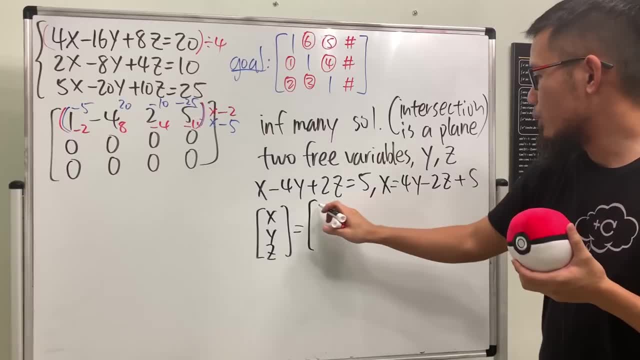 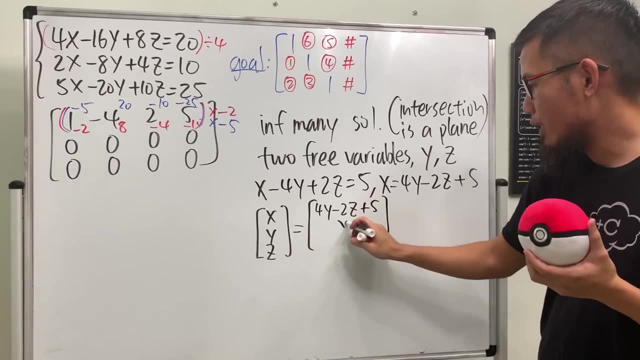 Well, x is what, x is all that. So we just put down 4y minus 2z and then plus 5.. And what's y? y is just y. What's z? z is just z. Why? Because they are free. 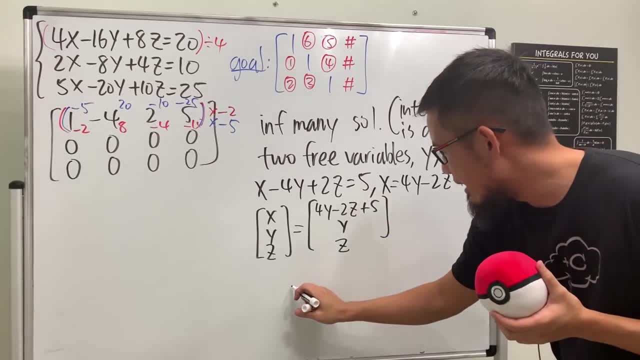 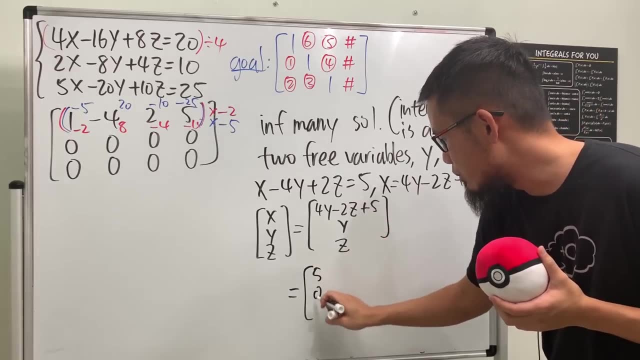 All right, And now we again just separate them, right And as you can see right here, let me just put down the constant first, which is just 5 and 0, 0.. So we write it as 5, 0, 0.. 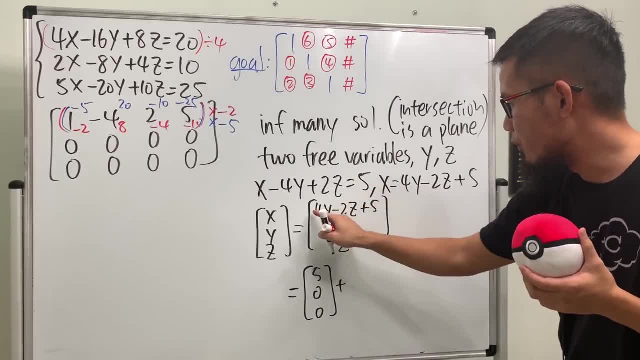 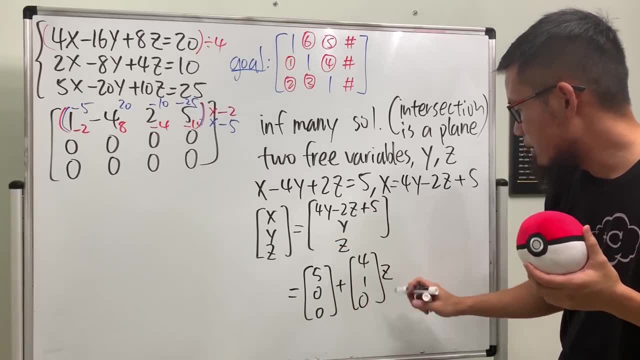 And then let's put down the term that has the y, So this is 4 and 1.. And then no y here, So it's 0. And then we have this factor times y And lastly just put down the 1 star z. 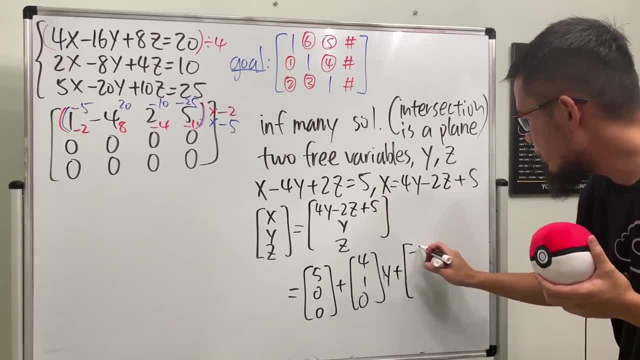 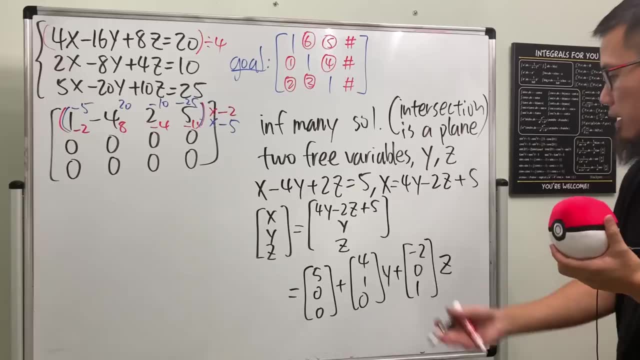 So this which is going to be negative: 2. And there's no z, So it's 0.. And we have 1 z, So that's pretty much it. That's how you can represent your solution. So again, this right here. 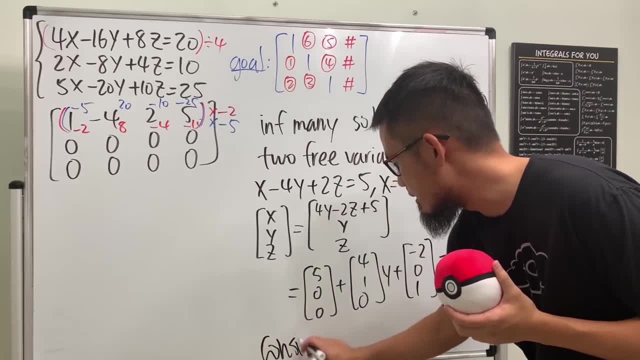 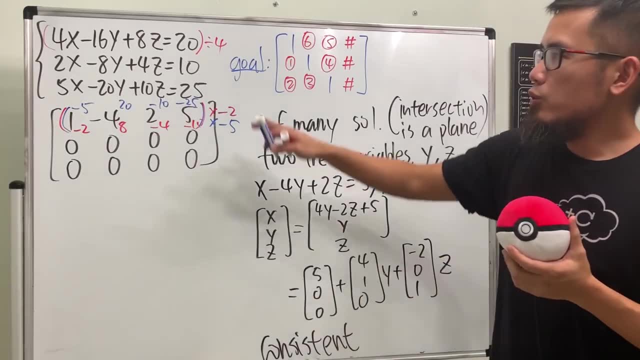 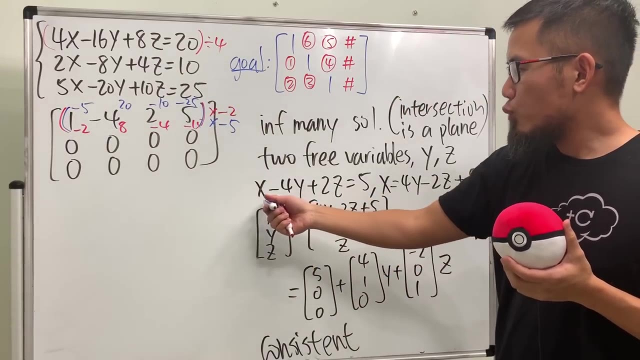 because we have solutions. So this right here is a consistent system of equations. Now, one thing to note is that remember from calculus 3, or maybe just like a general or pre-calculus class or whatsoever, if you want to grab this equation.